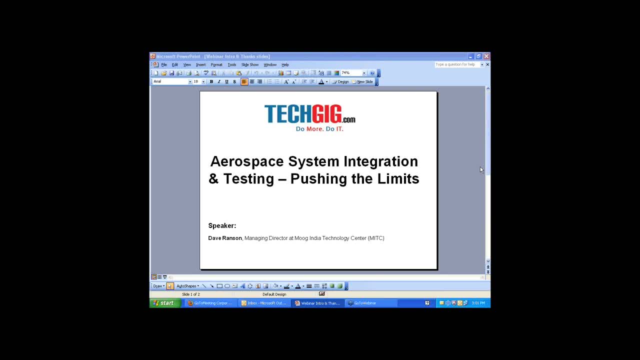 Nansen's concern here today. And finally, I'd like to challenge Mr Sean to stop the panel and at least the next panel with several more questions. So anyway, here we go. OK, So today I'm just going to go to. now to the audience. 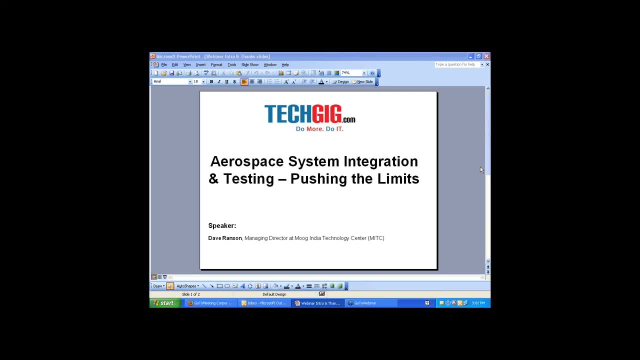 Could you expand on those three questions? There you go. OK, So we're in the room now along with the two live presenters, And, of course, there's three separate questions. Okay, Here we go. I'd like to make this time valuable for each of you. 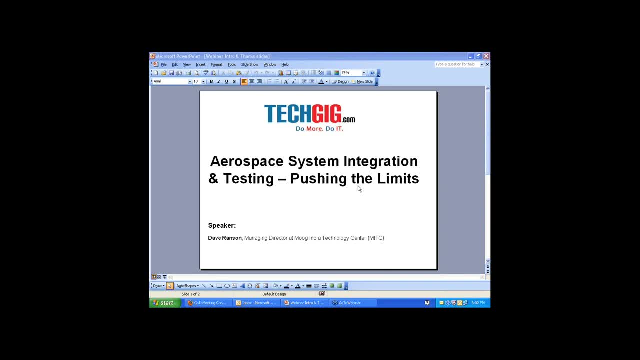 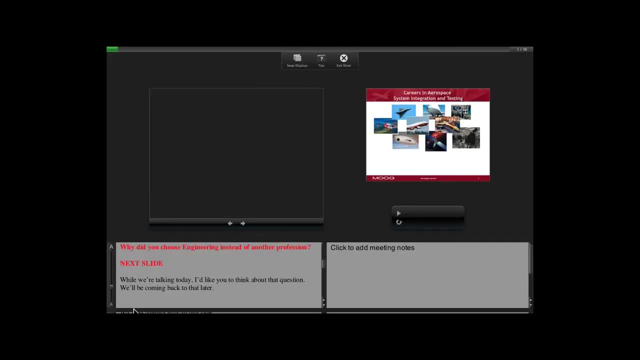 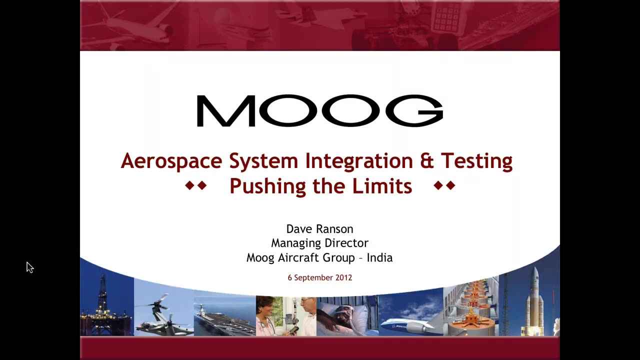 I'm looking forward to sharing a little bit about the aerospace industry and also about possible careers in aerospace. Today, we're going to focus on aerospace systems and integration, and the testing pushing the limits. Before we start, though, I have a very important question for the engineers and the engineering. 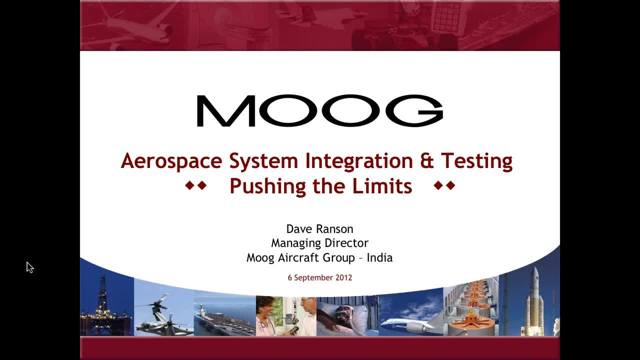 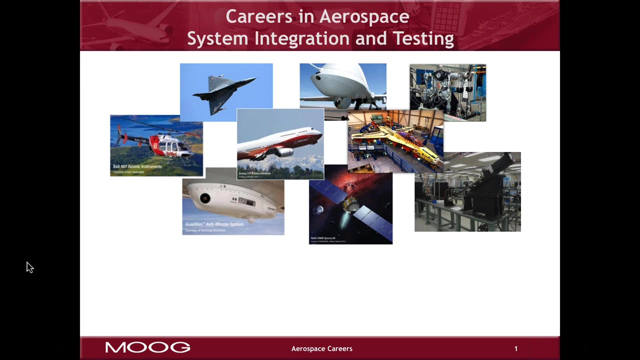 students listening today. Your answer to that question could have a profound effect on your future. Why did you choose engineering instead of another profession? I'd like you to think about that. while we're talking, Careers in aerospace To get us started, I'd like to give you some context for our discussion. 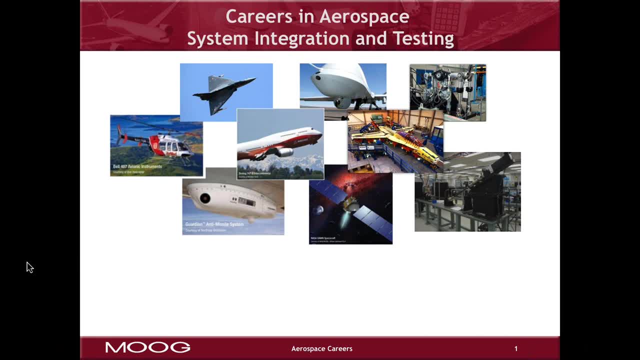 During my 30 years of aerospace experience, I've been involved with four different aerospace companies and I've enjoyed being with each of them. I'd like to share some of the things I've learned. Also, I'd like to talk just briefly about Moog, the company I'm with today, to give you 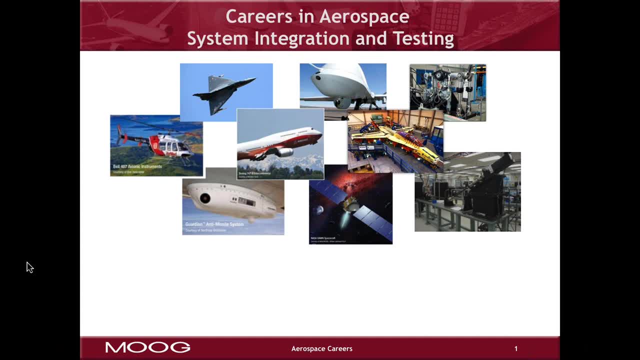 some understanding of the company. It's about 11,000 employees worldwide in 28 countries, $2.3 billion in sales US last year and probably over $2.4 billion this year. Moog is a worldwide designer, manufacturer and integrator of precision motion control. 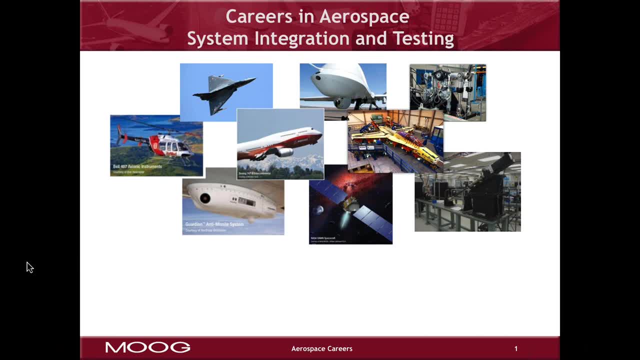 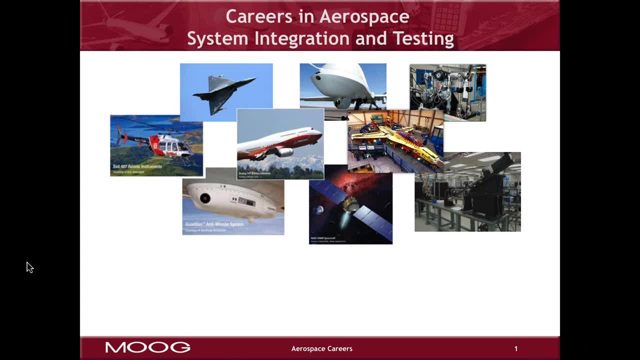 space vehicles and even to the retractable dome at Wimbledon. While we're waiting for the next slide to come up, I'll just…. Aerospace is a challenge because it brings together key engineering disciplines to develop complex test systems And specifically today, we will be talking about the extreme demands of aerospace and 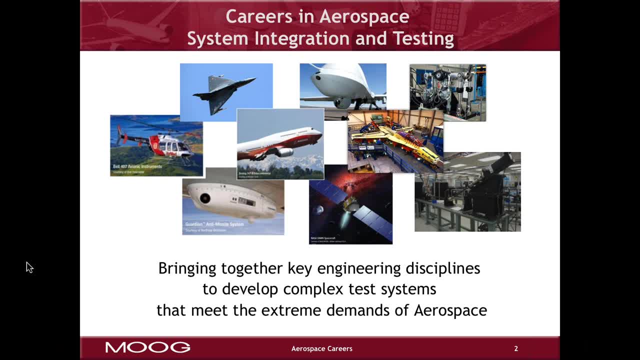 the complex test systems that support it. In aerospace, the drive is always for faster, lighter, stronger and less costly purpose, So a lot of the science and technology that we do at aerospace is making sure that we are building the best preparing and think and using the best technology to establish the 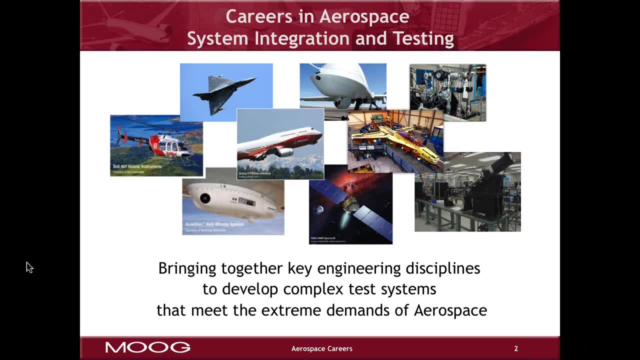 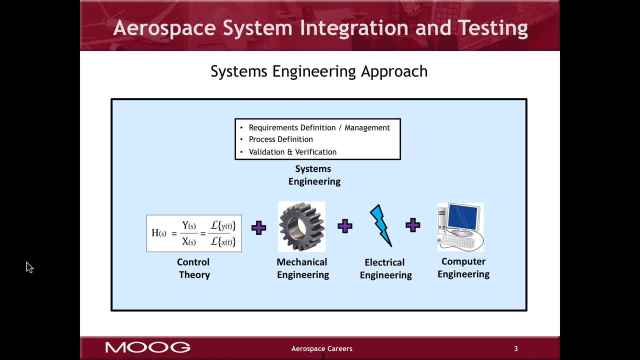 best possible and efficient performance for your horsepower, costly, in extremely cold and extremely hot environments. It's never an easy job. It requires engineers from almost every domain: mechanical, electrical software. It requires control theory, All of these working together toward a common goal using a systems engineering. 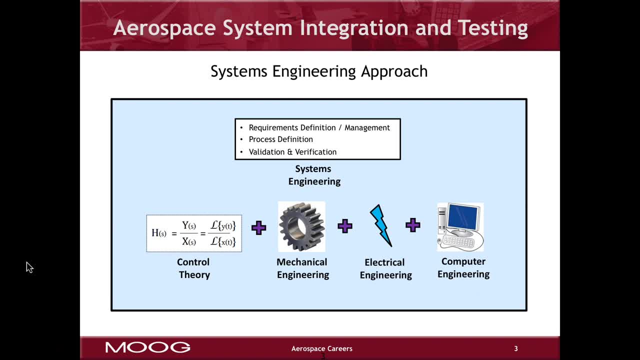 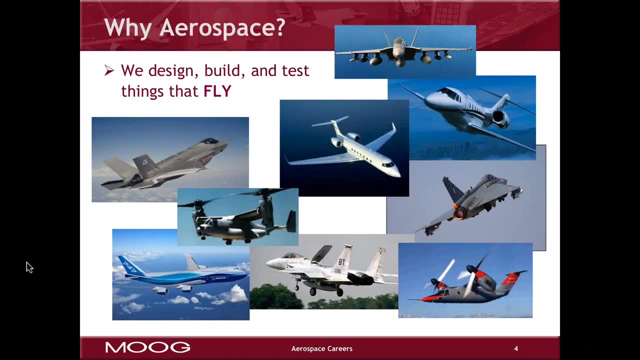 approach. So let's go back to the question I asked you earlier: Why did you choose engineering instead of another profession? Your answer to that question will help with this next question that I'm posing: Why would you choose aerospace? Aerospace is not for everyone. We'll come. 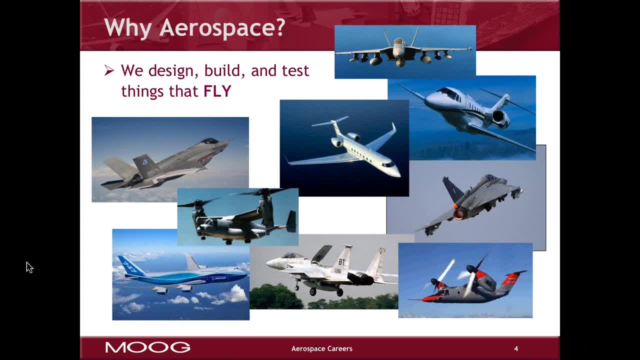 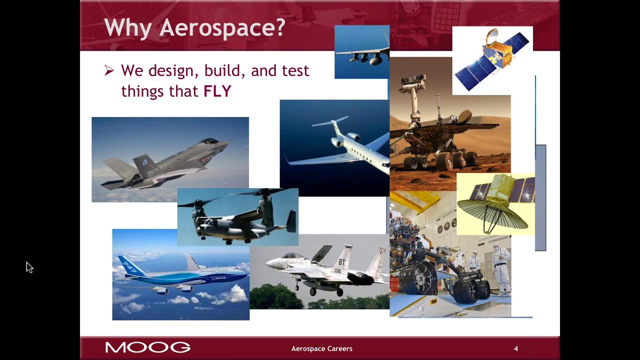 back to that, but first I'll tell you why I have chosen aerospace as my career. First of all, I love the fact that we design, build and test things that fly. There's more than that. Second, we design vehicles that can go anywhere. On the next slide you'll. 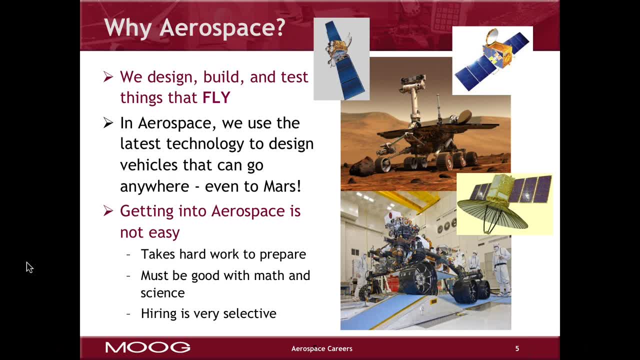 see vehicles that have even gone to Mars are part of the aerospace business. Now, getting into aerospace is not easy. It takes hard work and you have to be good with math and science. Hiring as a result is very selective because there are just a few positions available and many people interested. 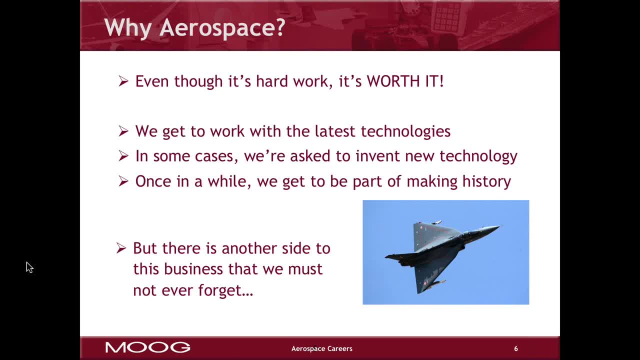 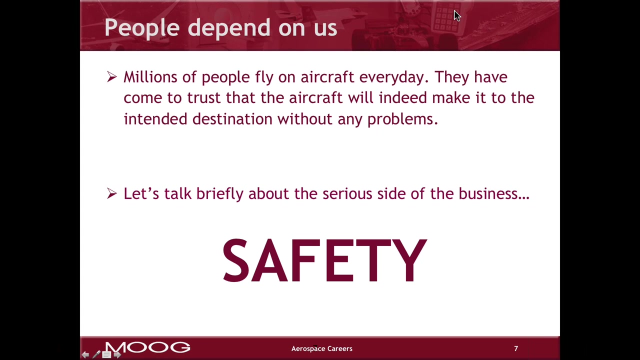 but it's worth it. We get to work with the latest technologies. In some cases, we're even asked to invent new technology. Once in a while, we get to be part of making history, For instance, the ground-breaking LCA light combat aircraft that India developed and which Moab was a part of. 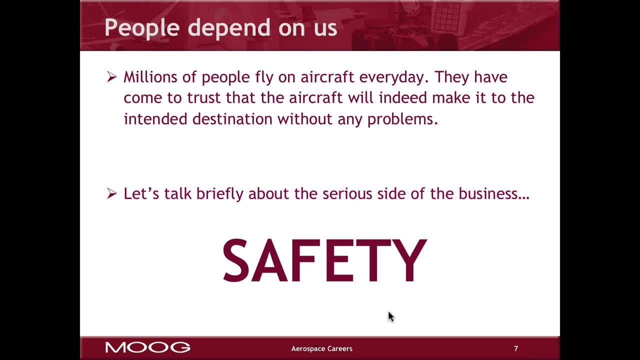 Let's talk about a serious side of the business. Every day, millions of people fly on aircraft, And they've come to trust that the aircraft will indeed make it to their intended destination without problems. And that's the serious side, because we are responsible, as aerospace engineers, for the 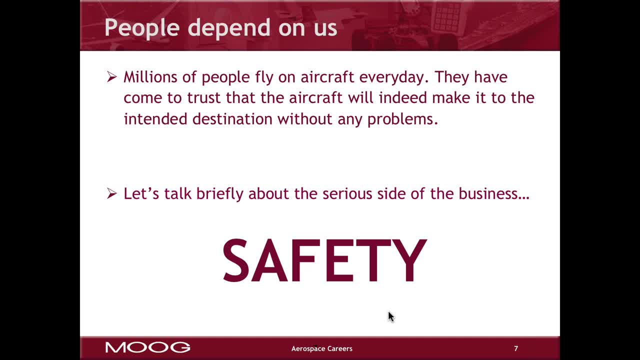 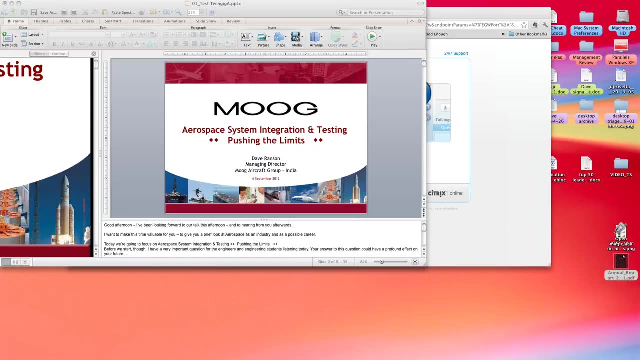 safety of the people who fly on the aircraft that we've designed. The first step we have to take is getting people to do it, and the first step is still one aspect that we have to take, And if you're not comfortable with it, then you have to do it. 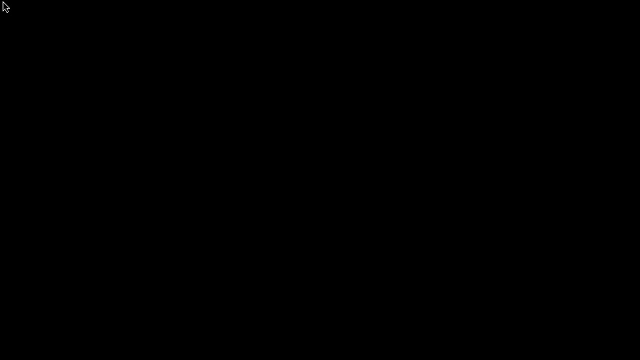 If you don't, you have to do it And you need to be able to do it. And this is an interesting stuff because you don't need to try really hard. It's just kind of a way for you to do it other ways. 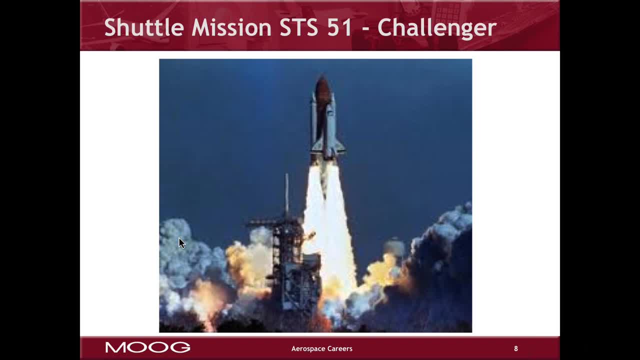 You're going to want to be able to do it, and you also got to have a really good understanding of how you're going to do it, And this is really important. And we're going to talk a little bit about this in a couple of minutes, but before I, 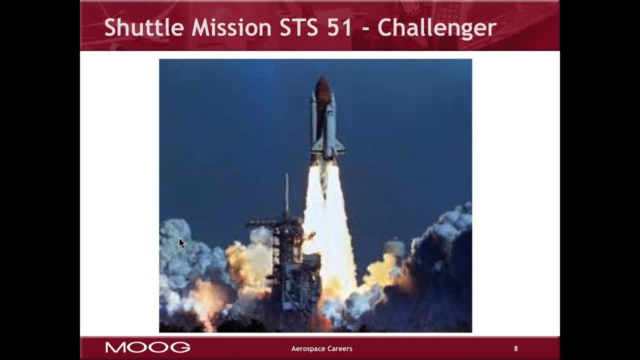 stop sharing my questions with you. I'm going to pop back in here just a little bit, Okay. This slide up here- this is the list- has been familiar to many of us for years. It's a picture of the space shuttle taking off from the Florida launch pad. 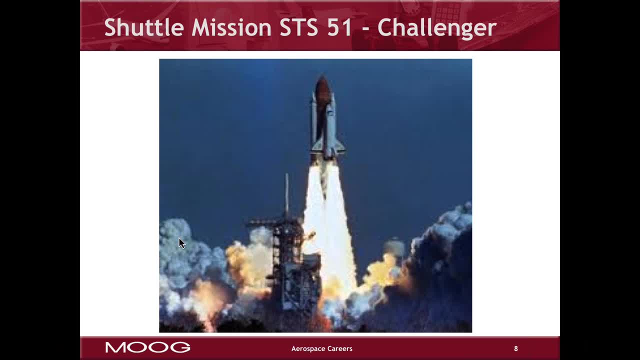 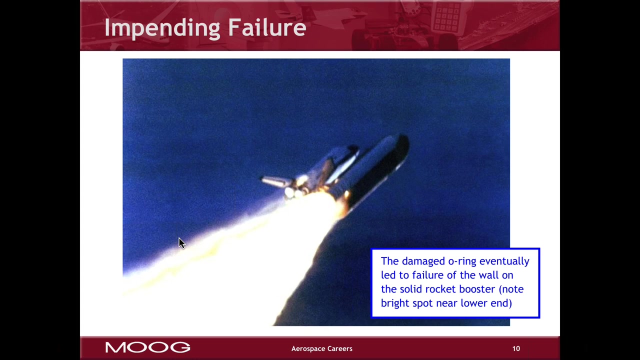 This is Space Shuttle Mission 51, TS-51.. No one knew that this flight would end in disaster, but it was in fact an inevitable surprise with terrible consequences, and it could easily have been prevented. O-ring damage noted as early as the second space shuttle flight, STS-2, was actually. 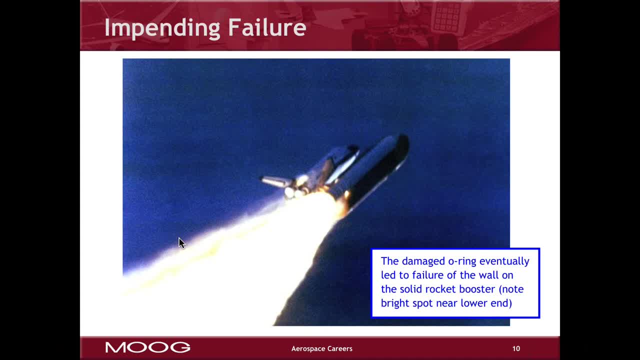 a criticality, one failure which should have grounded the fleet, But because of pressure to maintain schedule, the engineers were asked to run space special tests that tested the O-rings that had failed or were burnt at three times the pressure, and they made the decision to keep flying. 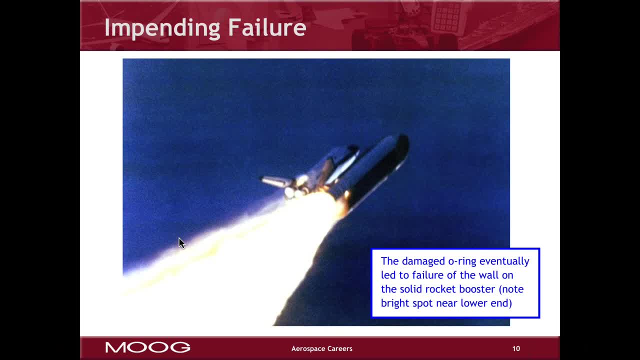 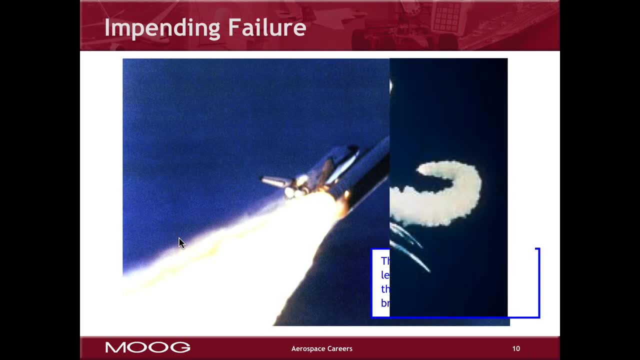 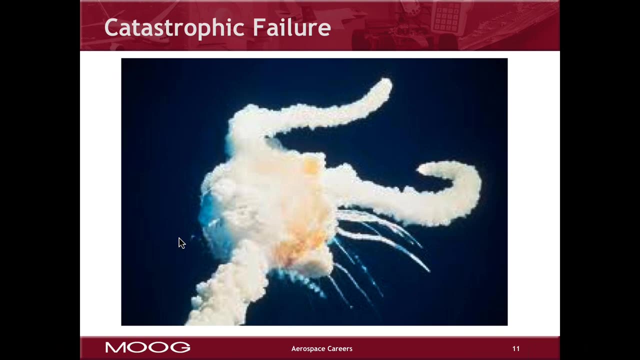 This decision was clearly against the operational guidelines for the program. In the ensuing flights, there were 12 additional instances of failure of the O-ring, of burning of the O-rings. The O-rings failed, but they were burned, damaged, and it was a question again: should. 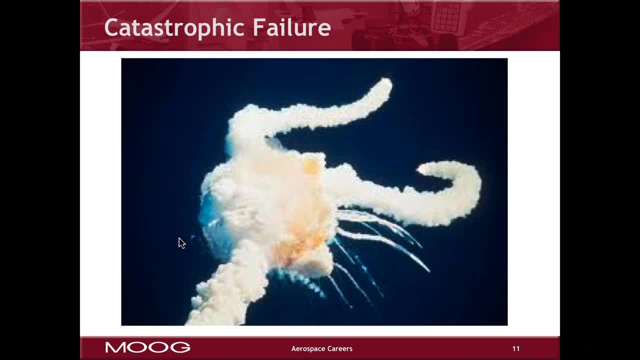 they fly. Each time, the engineers determined that it hadn't failed yet it must be safe. Unfortunately, on Space Shuttle Flight 51, the O-ring did eventually fail. You can see on the next slide that the solid rocket booster wall burned through and ultimately 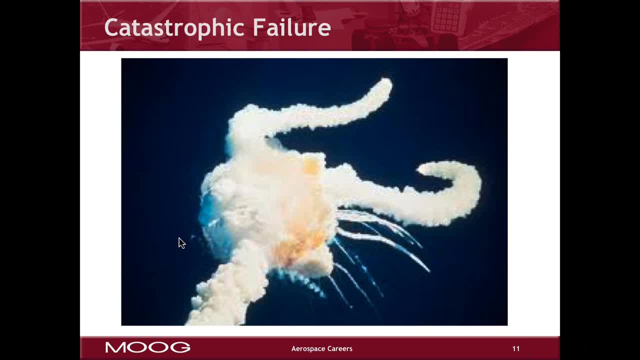 led to the complete failure of the mission. After the failure, the entire crew was lost and the two solid rocket boosters continued to fly while the shuttle wreckage plummeted to Earth. Now you may wonder why I bring up such a serious and sobering topic in the middle of a conversation. 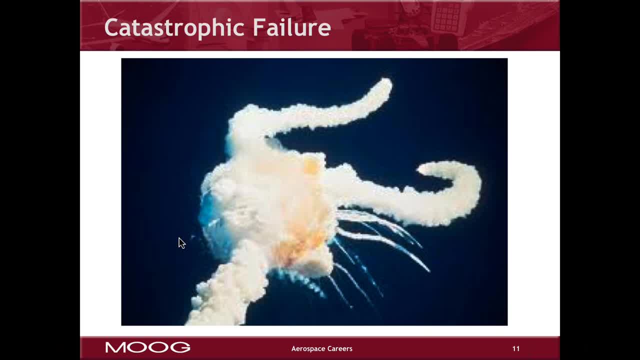 about aerospace careers, And it's this. Engineers in aerospace are sometimes called upon to make difficult decisions, And it's very important that anyone considering aerospace as a career should prepare to make difficult decisions. Ultimately, because of poor decisions on the space shuttle program, there were tragic results. 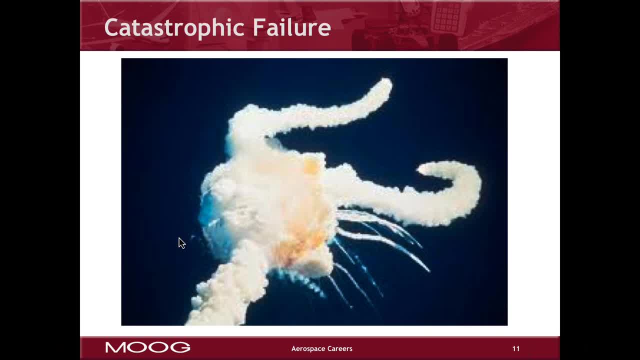 and the lives of hundreds of people were changed forever. Friends and family of crew members will never be the same. The engineers in aerospace are sometimes called upon to make difficult decisions, And it's very important that anyone considering aerospace as a career should prepare to make. 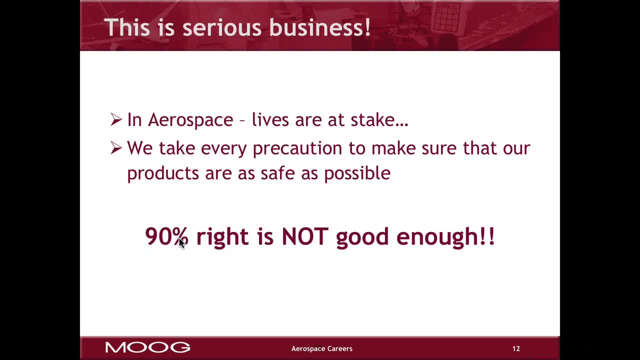 difficult decisions an aerospace career. you'll need to understand that it can be very demanding. in aerospace, lives are at stake and we take every precaution to make sure our products are as safe as possible. 90% right is not good enough, and that's why engineers are so important to this business. it's our job to design. 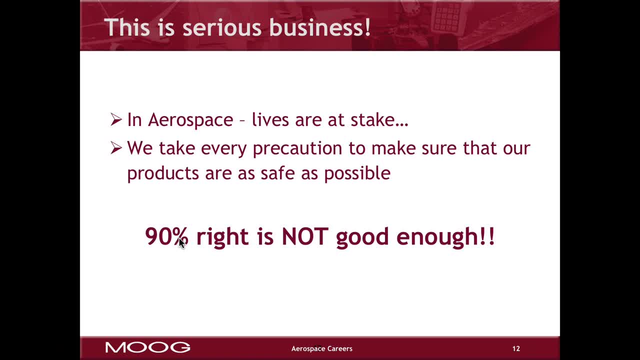 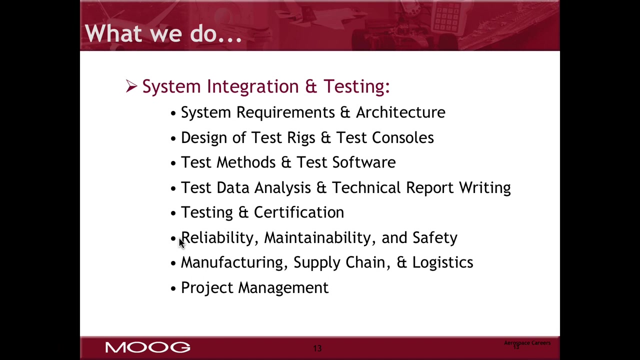 build and test products so that they're safe and, at the same time, to provide highest performance, the lightest weight and the best cost that we can. so let's talk about what you might do as a mechanical engineer or as an electrical engineer or as a computer software engineer in the system. 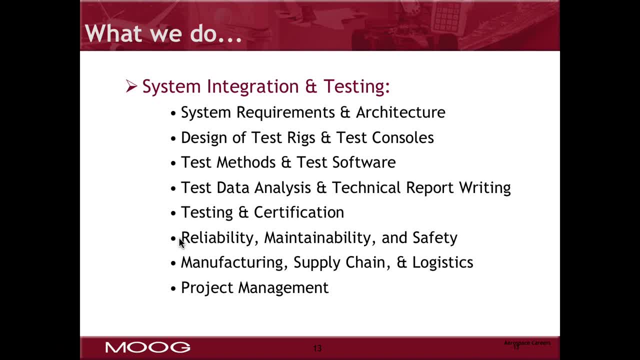 integration and testing process: arena for aerospace. the development process in aerospace takes eight major steps which, in the system integration and testing realm, require many different disciplines of engineering: system requirements and architecture, design, design of test rigs and test consoles, test data and analysis, technical requirements, testing and certification. each of these categories, you can see, require specific engineering skills. 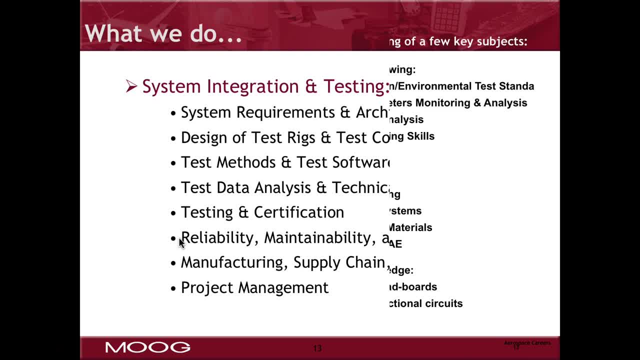 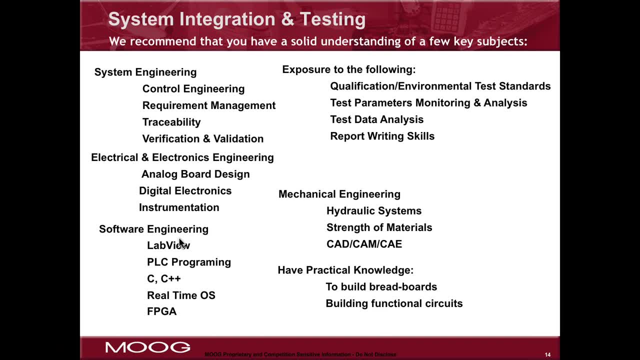 let's talk just briefly, as the next slide comes up, about what kind of preparation or understanding would be helpful to you in your career if you were to choose system integration and testing for aerospace systems engineering. engineering is a very important part of this, because the test system ends up being a complete self-contained. 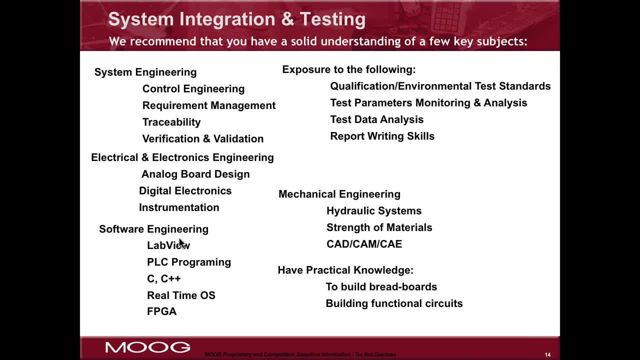 system. that requires the knowledge of control engineering, as well as some of the disciplines like requirements, management, verification and validation. other disciplines that are very important to this be electrical and electronics engineering in design and instrumentation, software engineers or the software that controls the tests, as well as mechanical engineering, understanding hydraulic and mechanical. 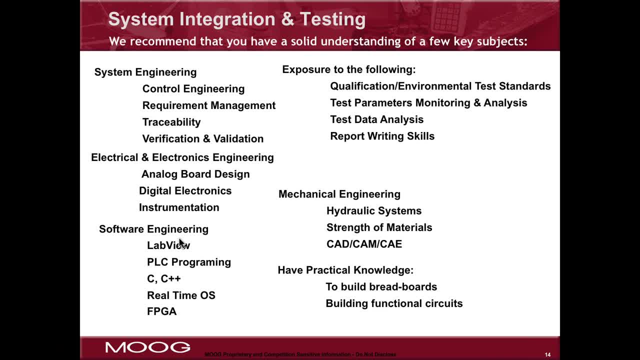 systems, strength of materials, having some of the tools like CAD and CAM, and having a product, practical knowledge of how to build circuits and breadboards for testing. now, all of these are important parts of your education as an engineer in system integration and testing. However, we don't expect you, as a young engineer, to come prepared with all of that. 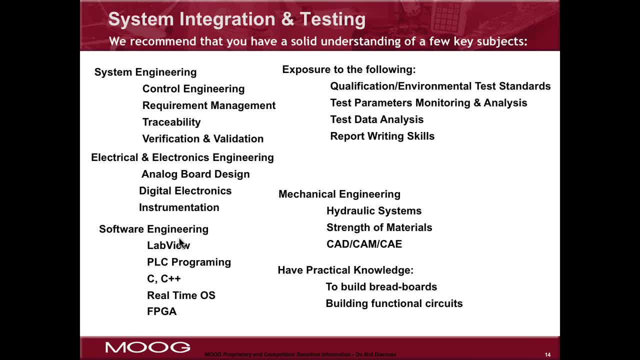 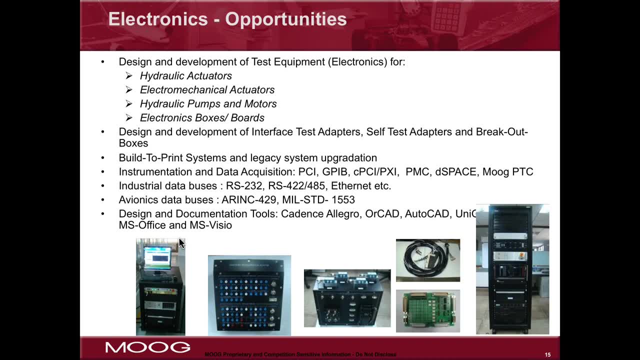 Many of the things we just discussed will be acquired skills. They'll be learning and growth during your career in an aerospace company. We're going to be going through a couple of slides rather quickly now that talk about the specific opportunities that you might find in different domains. 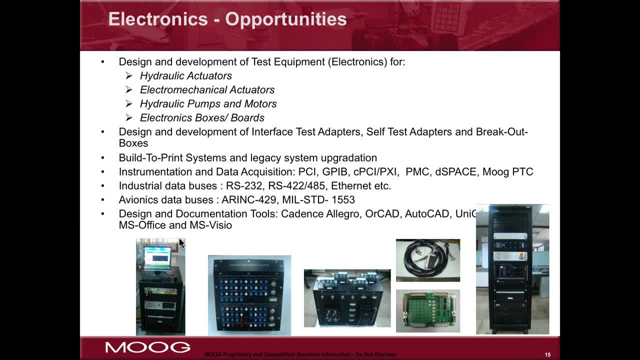 as an electronics engineer, perhaps, or a mechanical engineer. in the aerospace testing and system integration realm For electronics, there'll be opportunities for design and development of test equipment, Things that are important to understand. in the test equipment design would be hydraulic actuators. 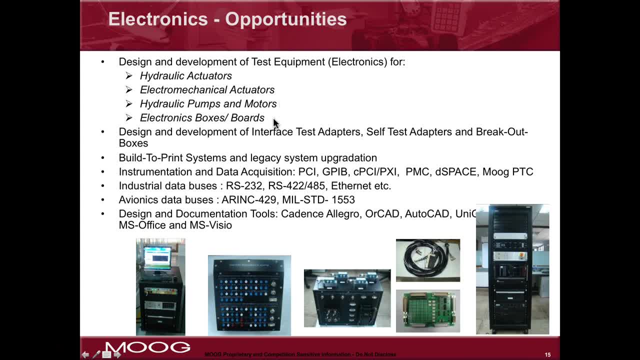 electromechanical actuators, pumps, hydraulic motors, electrical motors, electronic controls, the circuit boards and the controllers that they go into- All important to be able to design the optimum system to control a test system. The design and development of test interfaces. 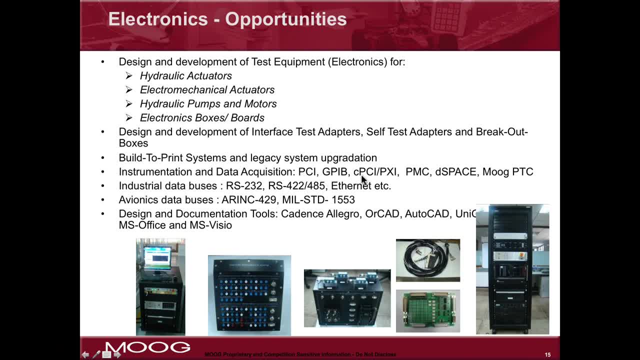 instrumentation and data acquisition is a whole other field, using various platforms and languages. Those are things you can get experience with in a lab, perhaps in a university. Some of the communication databases- RS-232, are familiar to many of you, but RS-422,, RS-485, and then the Ethernet, CAT-5 and CAT-6 protocols. 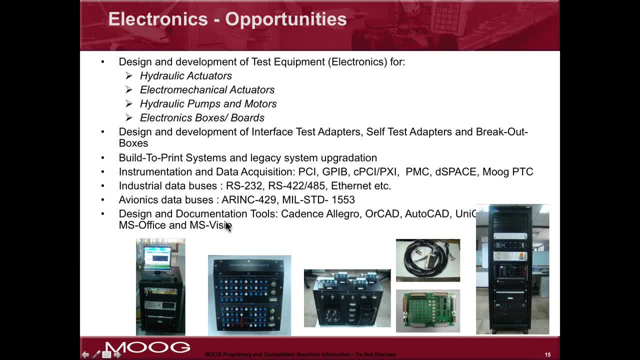 All important, but you don't have to come knowing all of this. A good knowledge base, Knowledge of the fundamentals, is your best bet. Avionics, data buses- which you probably don't see in the university, AIRINC-429 and several other AIRINC protocols. 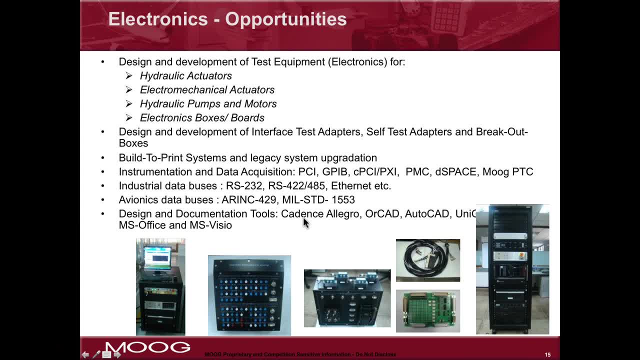 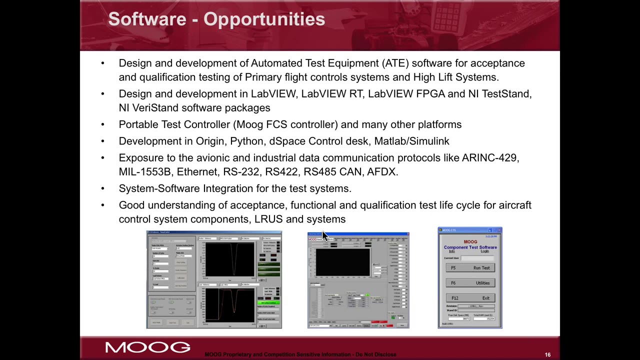 as well as MIL-STD-1553, are data bus protocols that we use often in aerospace And then for electronics. there are many tools that are used for electronics design, including Allegro and several other products. Let's talk about software. 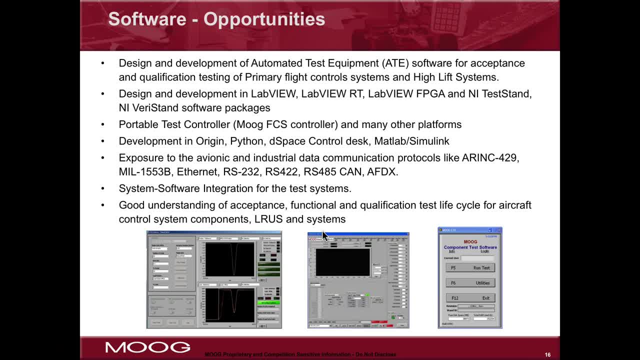 In software for the aerospace business there are two different domains. One is the embedded software that actually is designed for the flight control computer. The other is the software for the test equipment for the test system. We'll be talking about the second type of software technology. 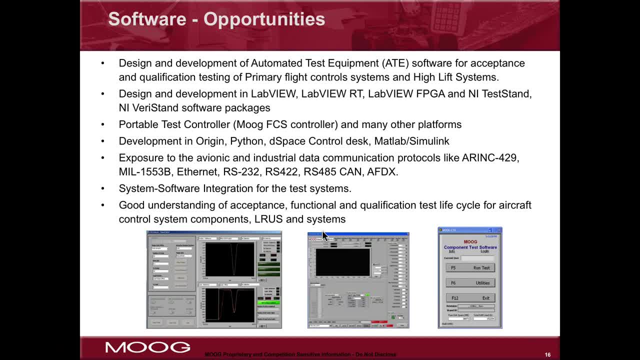 This is the type that's designed specifically for conducting tests of the electronics and the mechanical hardware. as a system For software, there are opportunities in designing automated test equipment, software, lab view and also languages. The first two types are the software for the lab, which is a very traditional software. 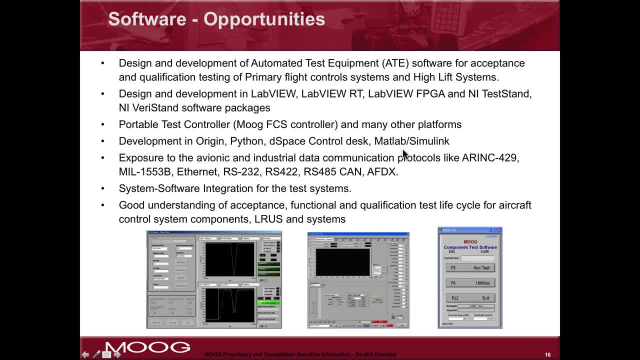 and then the software for the AIRINC-429., The second type being the software for the discussion module. The software for the discussion module is a very traditional software and I'll just make a short description. here is generally the software for the discussion module. 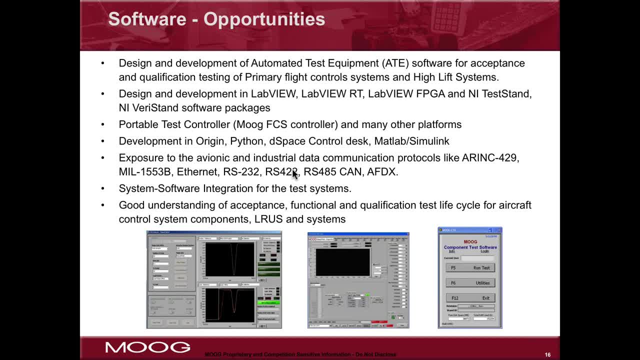 Let's see like ARINC 429 or MIL-1553, the commercial protocols, like RS-232, those will all be helpful. You have to know all of them. If you understand system and software integration, that will be a real help and that's something. 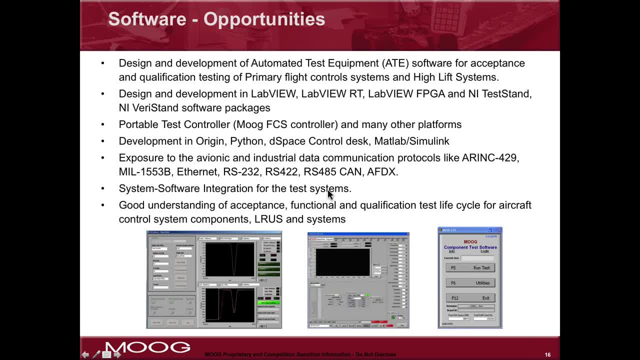 you can perhaps explore in the lab at the university. Ultimately, we'll help you get a good understanding of acceptance testing, functional testing, qualification testing and what those life cycles are about and what the control systems need to look like for those applications. 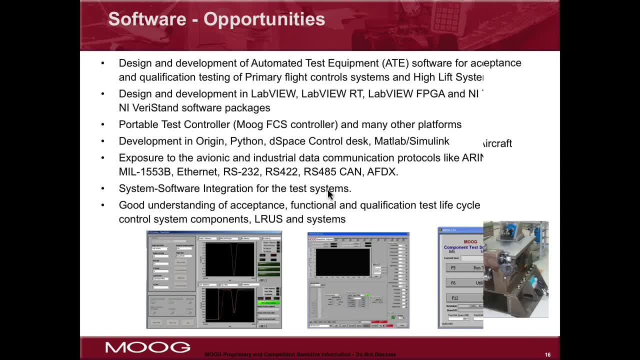 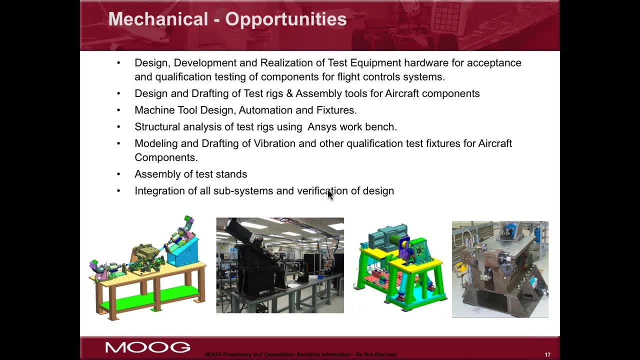 Ultimately again, though, two types of software in aerospace. the type we're talking about today is for test equipment and test systems. There's another type of software, embedded-based software, for the flight control computers, which Moog also designs, as do other aerospace companies. 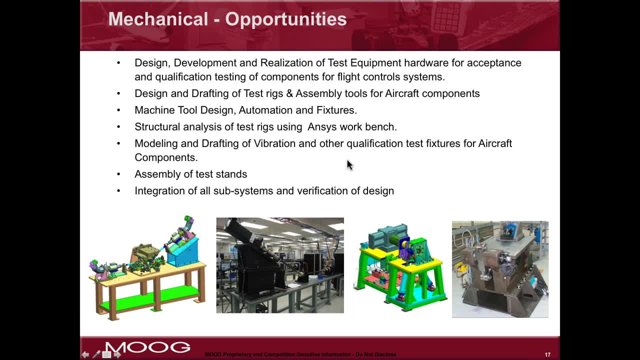 And we'll be talking about the software in our TechGig session next week. The next slide that comes up for you- I'm hoping you'll see it about now- is mechanical. For mechanical, the opportunities are primarily around the actual test fixtures. 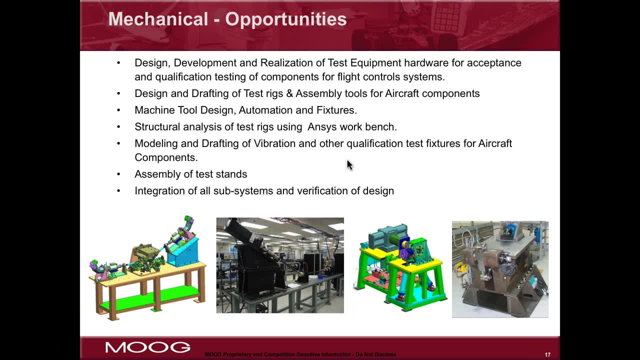 that are used to put the components through the most rigorous of tests, And a mechanical engineer might be called to design and develop a large test fixture for a geared actuator or a hydraulic cylinder or a system of multiple LRUs, which is line replaceable unit. 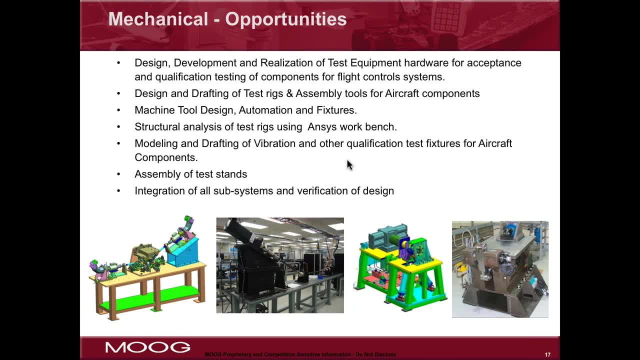 Many different disciplines go into that. There are all kinds of disciplines. There are all kinds of disciplines that are used to design and develop a large test fixture. They're all mechanical engineering related: Design and drafting of the test rigs and the assembly tools. 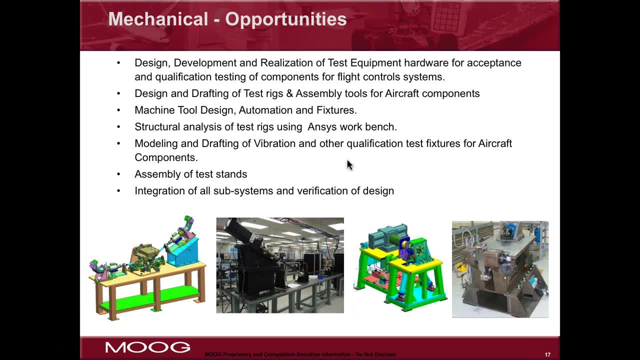 Also designing the fixtures that are used to manufacture the parts, Modeling and drafting of a vibration fixture or a special test fixture for production- All could happen under the guidance of a mechanical engineer. There's also a great opportunity to work hands-on with these test rigs and the technology that we're testing in them. 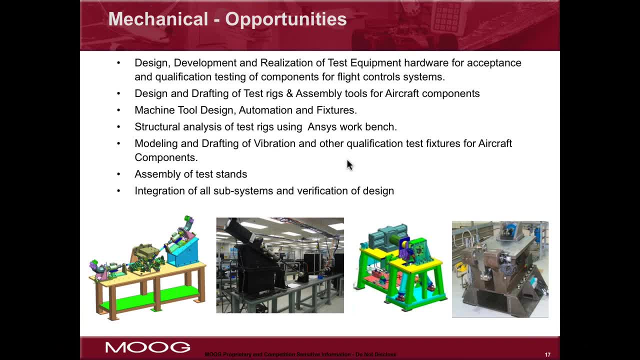 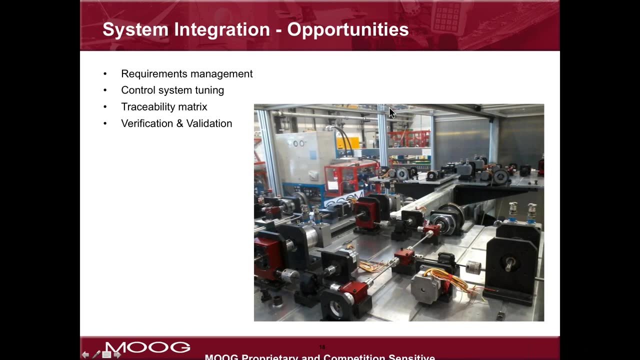 to work on the integration of the actual test unit that will go on in an aircraft eventually with the test equipment. We'll be going to another slide now and I think there may be a little bit of a delay, But the next slide is talking about integration. 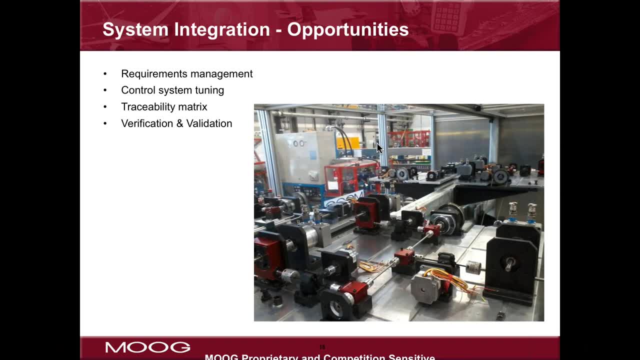 And I'll just talk a little bit about integration. The system integration and test domain is a unique in a unique position in the aerospace industry because it involves designing and developing and integrating an entire system. In many ways, the system integration and test domain is doing a smaller version of what the aircraft manufacturer does. 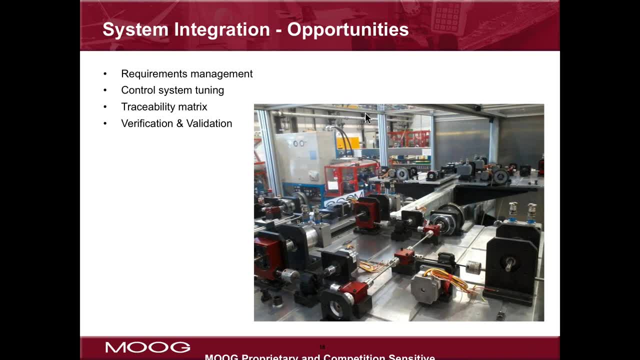 in creating a control system that acts in many ways like the control system on the aircraft. You should be seeing a picture now that has the title System Integration Opportunities And in this domain, the, the, the. the primary emphasis is on understanding the requirements of the system. 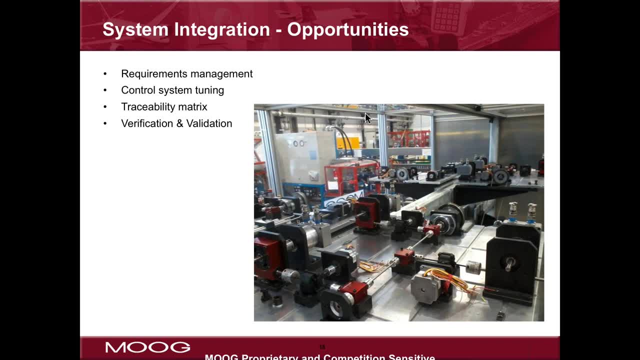 and then making sure, when all is said and done, that the requirements have been met, And that requires some very sophisticated engineering. in fact, Understanding the requirements upfront and making sure the requirements are realistic takes good engineering judgment, which is often developed over many years. 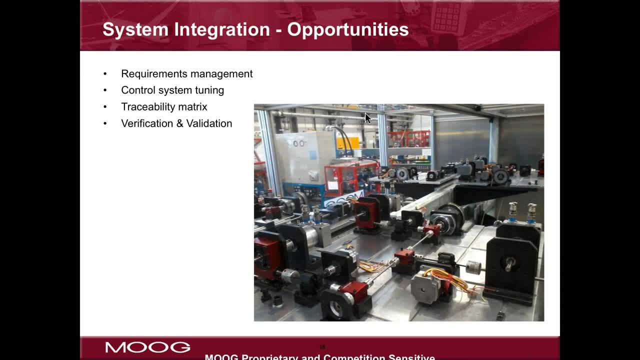 Learning to tune a control system- the spring mass damp damping systems that are present in any mechanical test system- takes some good basis in the knowledge of control theory and also some on-the-job experience. But when it's all said and done, the engineer who's responsible for system integration also is required to be able to 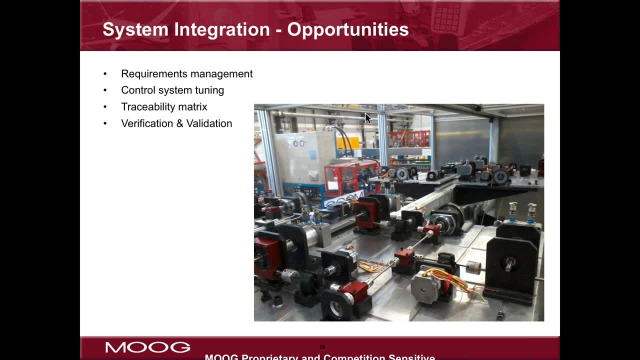 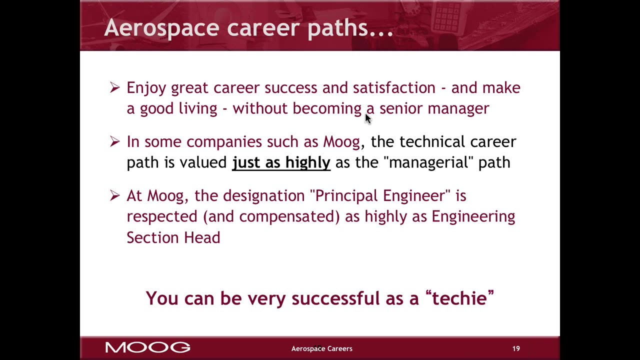 to document the fact that all the requirements were met, so that there aren't any surprise requirements that would actually cause danger on the aircraft. The next slide: we're heading towards a discussion of career paths specifically in aerospace, And I'd like to talk with you now just briefly about 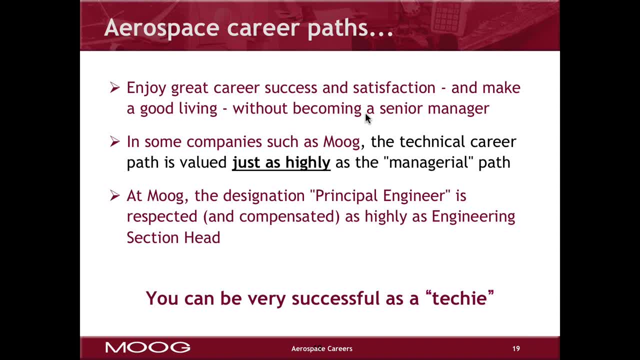 the, the difference between an aerospace career and perhaps another type of a career, still in engineering. Aerospace careers offer a unique opportunity because the, although there are, the aerospace field is much smaller and there are fewer people hired. there's a unique opportunity. 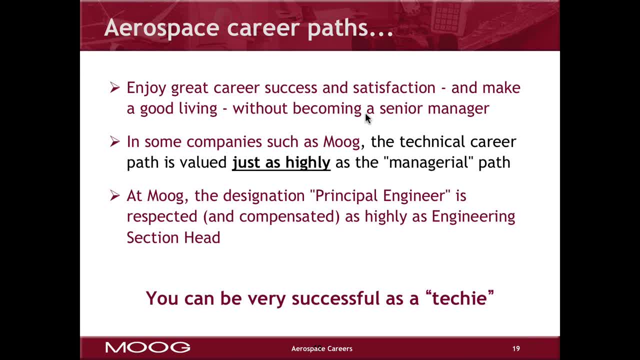 especially in companies like Moog in aerospace because the technical career path is valued just as highly as the managerial path. At Moog and in some other aerospace companies in my experience the designation principal engineer is respected and compensated as highly as an engineering section head. 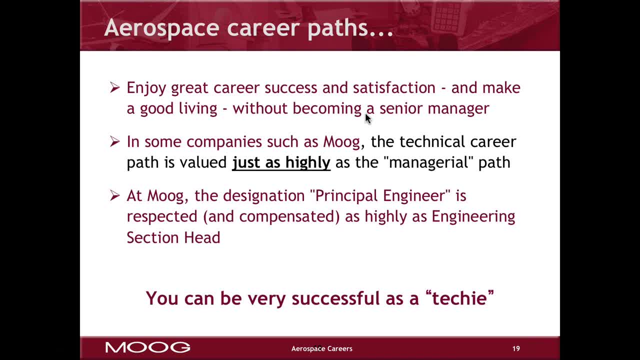 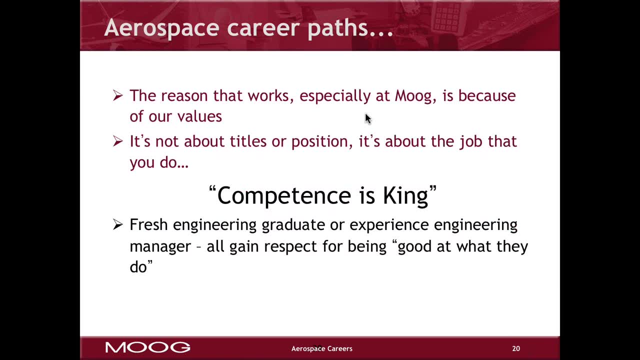 The message there is: in aerospace, you can be very successful as a techie. Now, the reason that works, especially at Moog, is because of values. The reason that works is because the most effective way to work together. 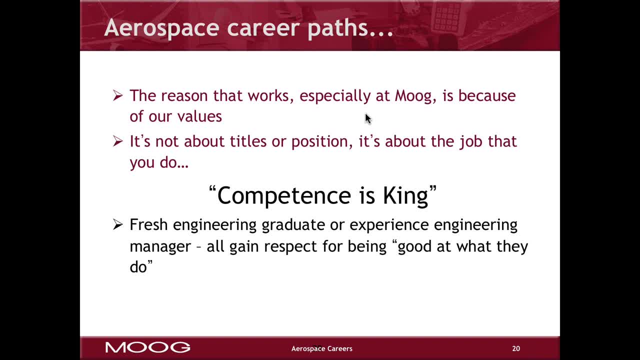 in a collaborative environment is not to worry about titles or position. The strengths of an aerospace environment in many cases is that it's not about competence or an experienced engineering manager. both gain respect for being good. 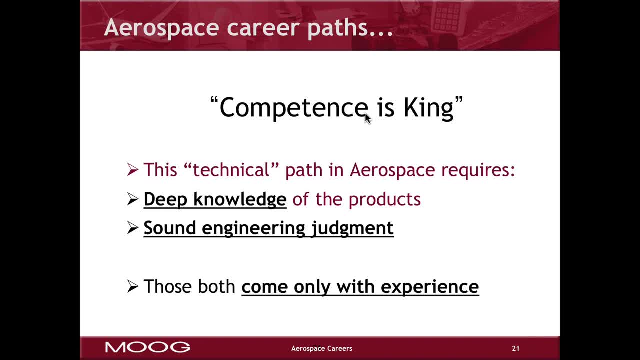 at what they do The other. There may be a little delay in the slide here, but the next path talks about the challenge of the technical path. It's not an easy path. It requires the products and it requires engineering judgment, And both of these come only with experience. 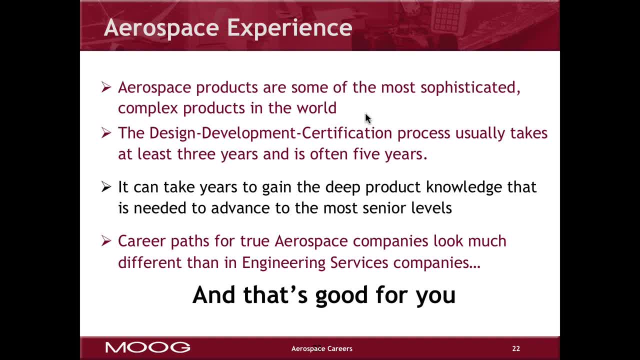 Now. aerospace products are some of the most sophisticated, complex products in the world. The process that we use to design, develop and certify those products usually lasts at least three years, and is often five years. That seems like a long time, especially in aerospace. 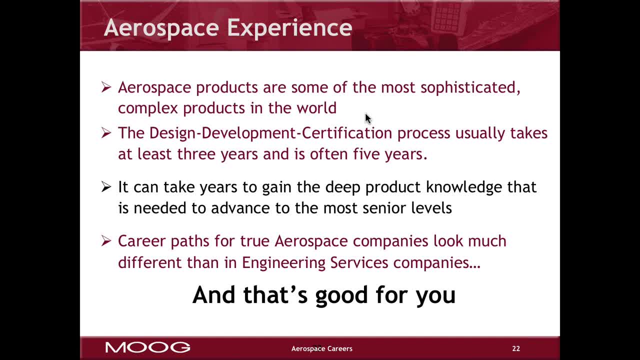 In a world today where products have development cycles that are measured in weeks and months, not in years. But it's the nature of the business, because there is so much new technology required and because there is such a need for safety and for being absolutely sure the product is safe. 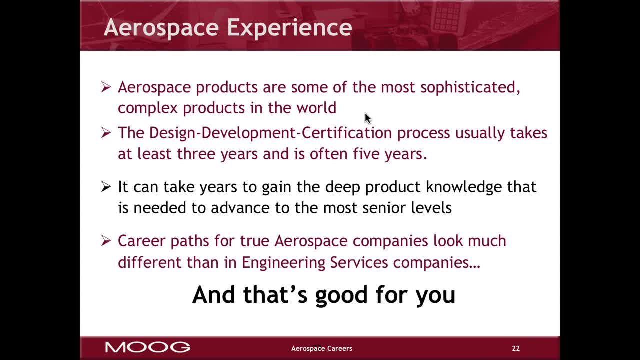 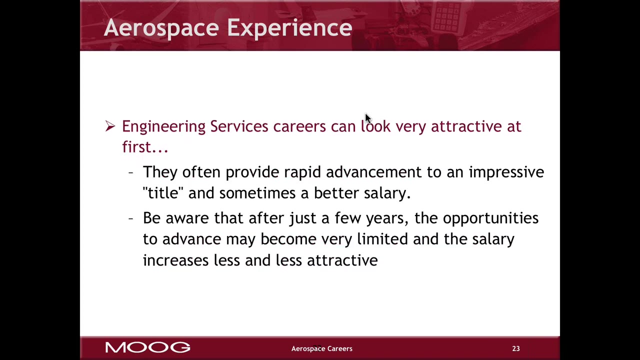 that it can take years to gain the deep product knowledge that you need to advance to the most senior level. So career paths for true aerospace companies look much different than in engineering service companies, And the message is: that's good for you. Why is that? 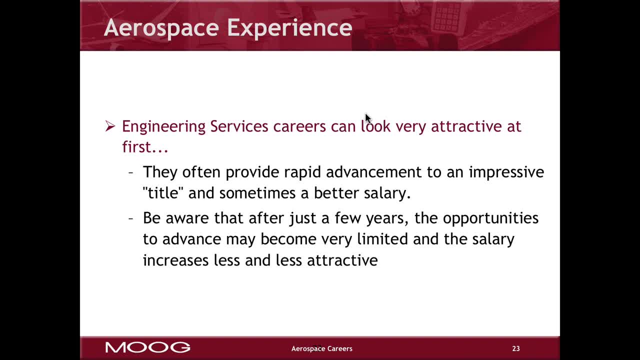 I'll put it in these terms: Engineering services careers can look very attractive at first And in fact they can be very attractive at first. In fact, there are challenges and that's a good career path for some, But I'd like to offer that for a very few in the audience. that may not be what you choose. 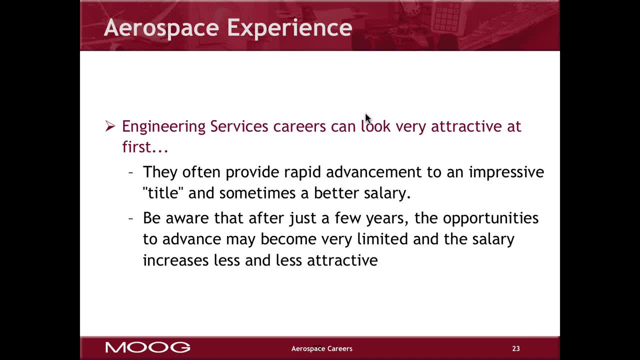 An engineering services career may not be right for you. In engineering services you often see rapid advancement and often an impressive title with a good setback. But if they do do well for the project, you may want to look at creating a fonctionne career path. And I'd think that's rather the cybersecurity and security lead. I would also like to take some time to emphasize that the career pathway may be very interesting. Let me just give you one more thing. If you are successful management teams, you already know that at some level angels will pick up the apl�. onvetting and 묻hing rollout from surface technology And if you're separate, once you're in this company you will not even notice your introduction só to something as creative as having a visual interface. And in any case, you'll be listening at your心 list a couple of times. 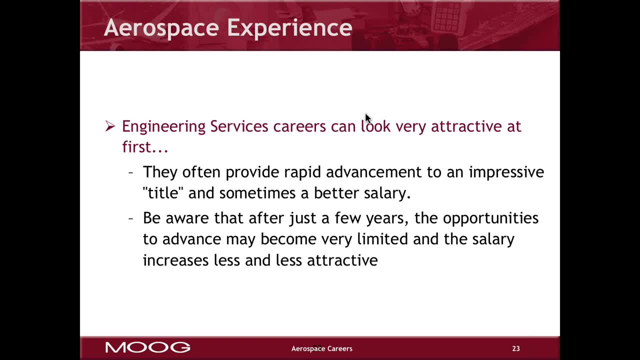 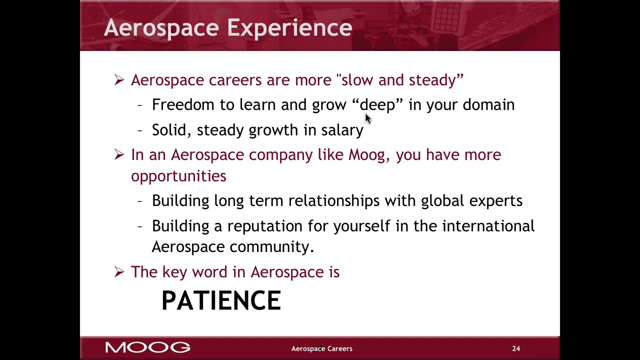 My personal opinion. reviews with factory obviously are important. If anything, it's because you can give yourself a little bit of a stutter when then you have to make sure the Aerospace careers are more slow and steady, I guess that would be the phrase I would use. 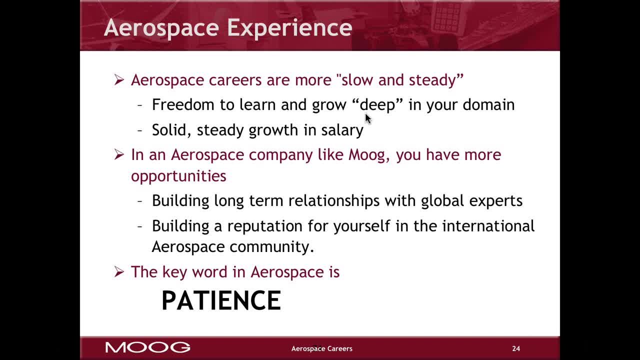 An aerospace career will start out with a competitive salary in the region and there will be the freedom to learn and grow deep in your domain. as you grow in your career, There will be solid, steady growth in salary, But because of the need for significant experience to get 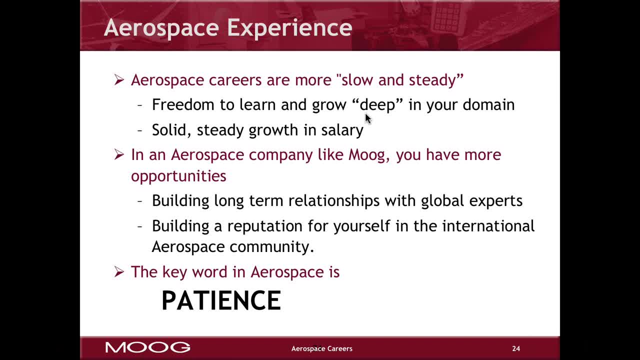 In your responsibilities. I would offer one particular benefit that I've seen and experienced myself In an aerospace company like Moog. you have more opportunities for building long-term relationships with global experts Because, instead of being one among thousands, you're one among a smaller community. that 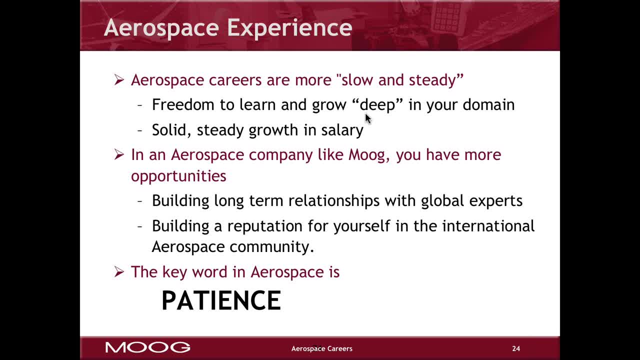 is actually a global network. The other thing is that you are free to build a reputation for yourself and, in fact, you will be building a reputation for yourself in the international aerospace community Because it's a global business, A global business with a relatively small community. 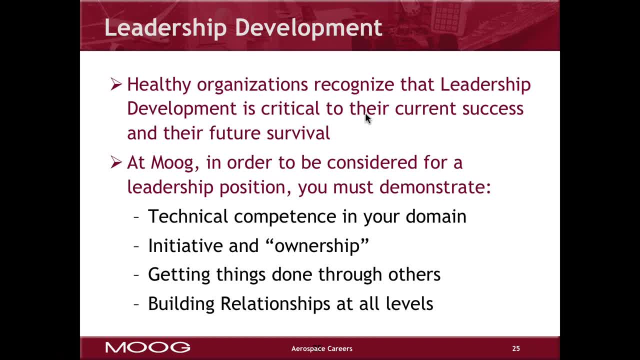 The key word in aerospace is global. The key word in aerospace is patience. Now, along with that patience comes some great benefits: The ability to learn and grow, Satisfaction in your career. that perhaps is not available to everyone in some of the other communities. 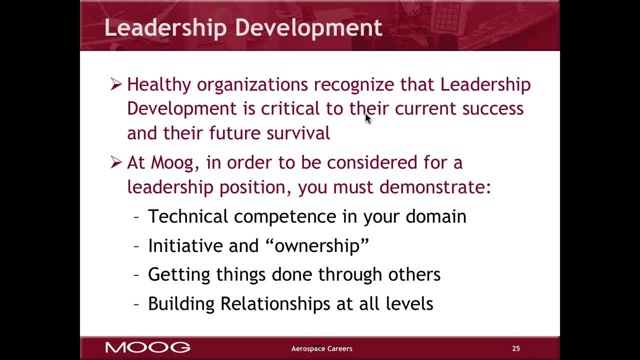 At Moog and in other aerospace companies to move into leadership. there are going to be some specific things we look for. We realize that leadership development is critical to our success as a company and to our survival in the future as a company. 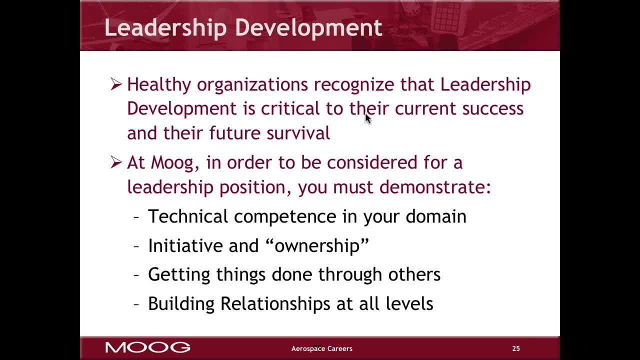 So we're looking for emerging leaders who demonstrate four important characteristics, And the number one is technical competence in your domain. In aerospace, the expectation is that you will be very good at what you do in your technical domain So that, when you get to a position of leadership, you will be able to make wise decisions. 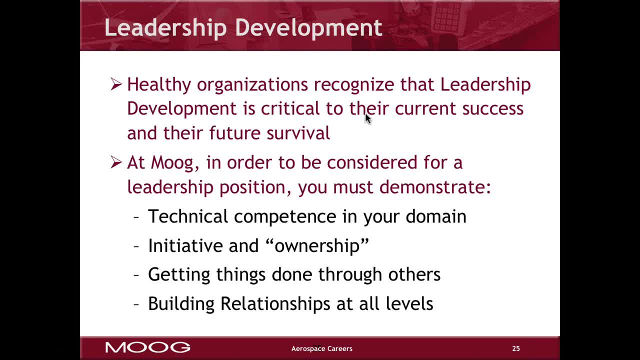 Because ultimately, as a senior leader in aerospace, you'll be asked to make some very difficult decisions that require deep knowledge and solid engineering judgment. So technical competence- That is the first requirement. The engineers who bring that to the table are then asked to show initiative and to show 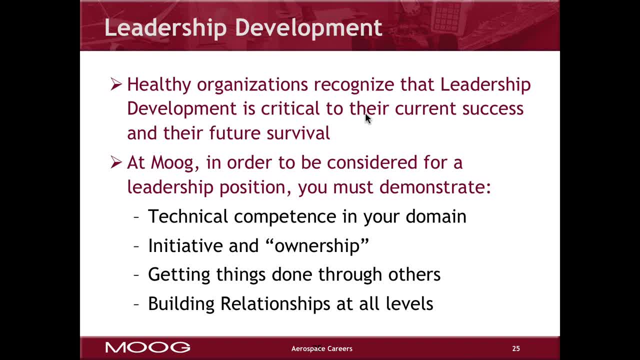 ownership, Meaning if there's a project that needs to be accomplished with a team that the engineers on that team all believe it's their job together to get the job done, They own it. Another thing we look for is getting things done through others. 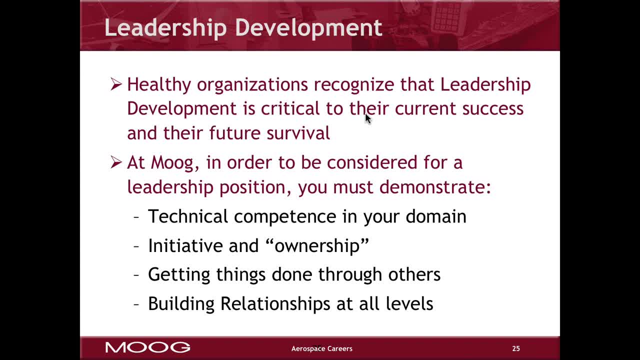 And that's a combination of being good at planning and delegating, but also at being very good at working together with a team, working with others. And then very important for a global enterprise, as most of the aerospace corporations are these days, is being able to build relationships at all levels. 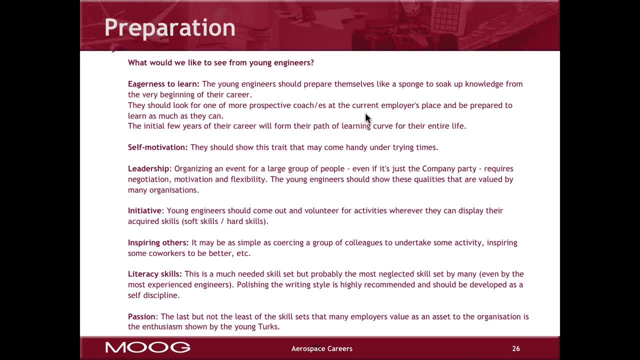 In the aerospace organization, a young engineer will be asked to interact with his peers, with his supervisor and perhaps with seniors several levels above, as well as others that are reporting to them, And they're expected to do that with respect and dignity at all levels and with the courage 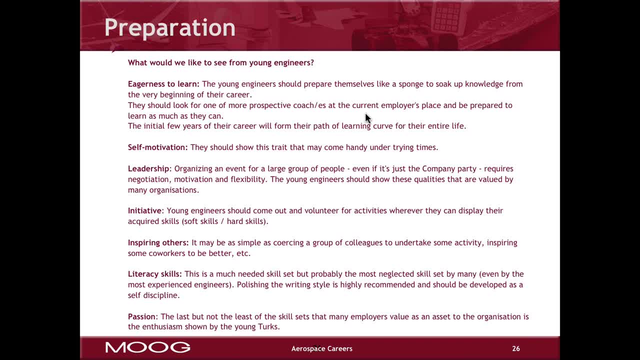 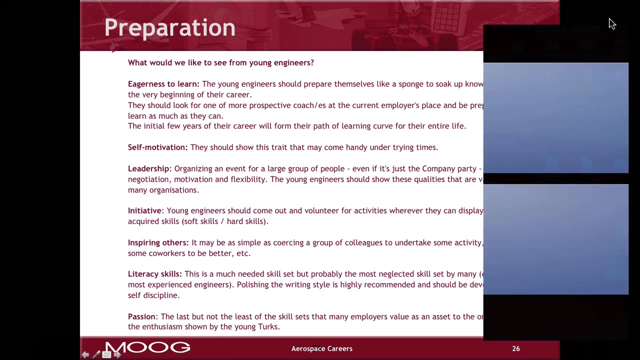 to say the right thing, to say the truth in all circumstances. So the next page is: I apologize for the fine print, but it has some really good pieces that we'd like to have you thinking about as you prepare for approaching an aerospace company for a potential job. 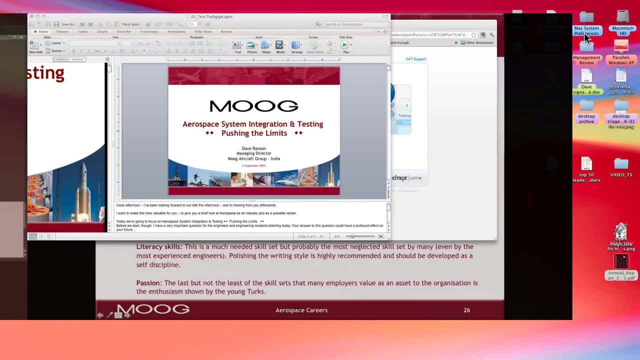 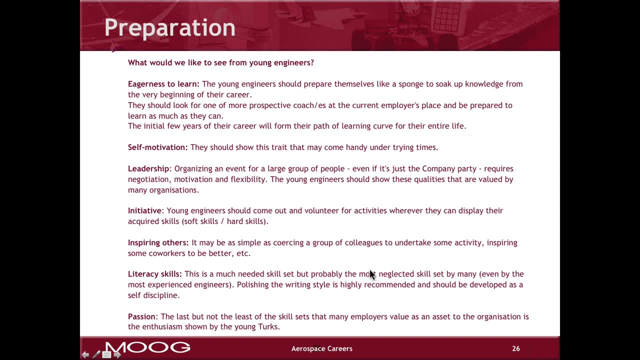 What would we like to see from young engineers? We would like to see An eagerness to learn. We'd like to see someone who really enjoys the prospect of learning and wants to grow, Because the initial few years of a career are very important- learning times and in 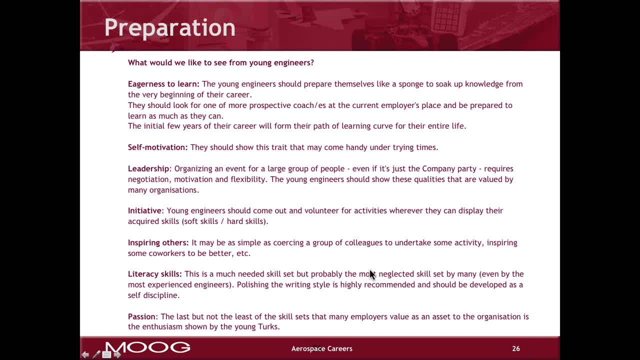 fact set the pattern for learning through the entire career. We'll come back to it later, but learning never stops in aerospace. Self-motivation That goes along with the initiative and ownership that I mentioned in the previous one. We'd like to be able to see that you really are taking action to make things happen. 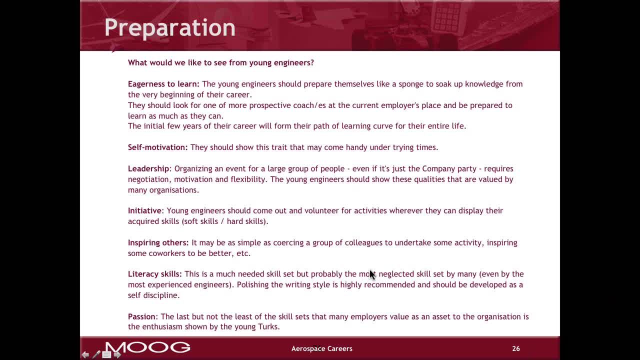 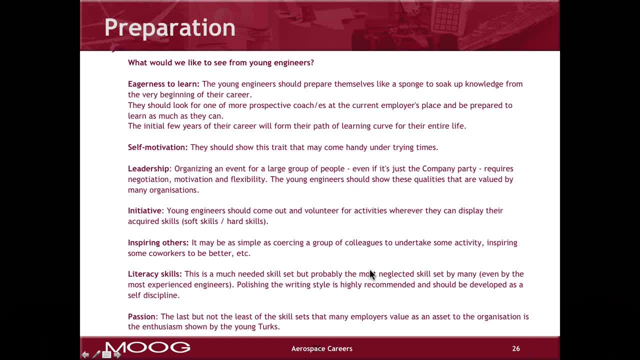 Inspiring others. Inspiring others to be better by example and by encouragement is a very important thing. Is leadership by example, not by coercion Literary skills. What we mean there is the ability to communicate verbally is important. That's a great thing. 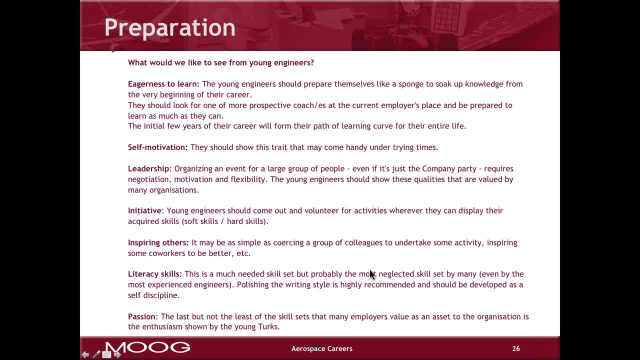 That's a great thing. That's a great thing. But written word, in either emails or reports, is very important, And so if you can polish that skill as you're going through your engineering education, that will be a very important skill for you to bring. 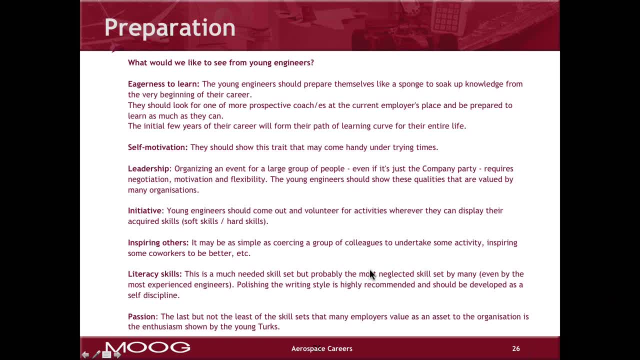 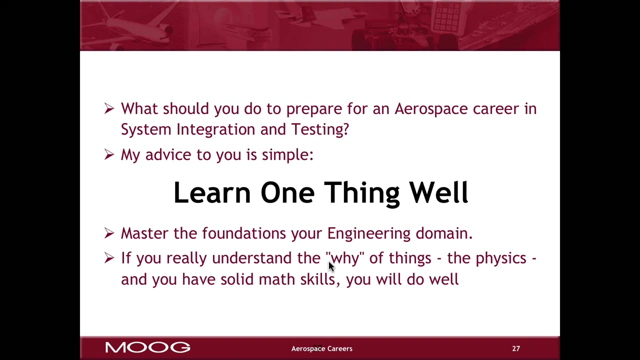 The last piece, perhaps, is the most important one, though. Ultimately, in aerospace, we love what we do and that's what drives us to excel, And we really do look for young colleagues who bring that same passion. With all of that said, as the next slide comes up, 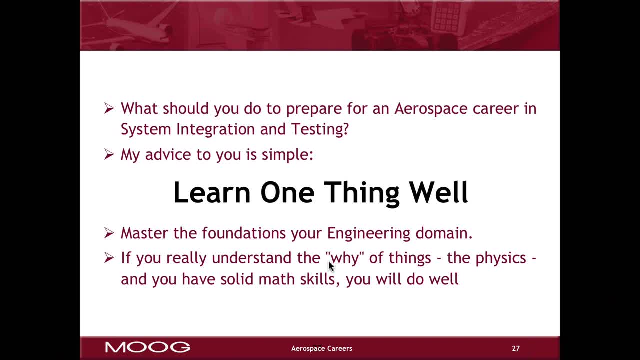 I would encourage you, with all those things we've listed, that it's most important in your preparation for a career in system integration and testing, to do this one thing, and that is learn one thing well, Don't try and learn it all. 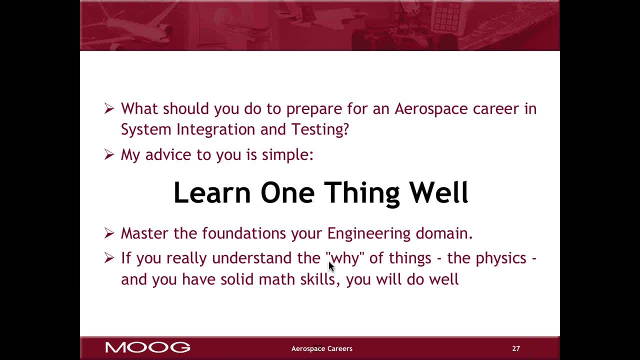 Master the foundations in your engineering domain. If it's electronic, If it's electronic engineering, learn the basics. If it's in mechanical engineering, learn the basics In computer engineering. you guessed it. I'm going to say learn the basics. 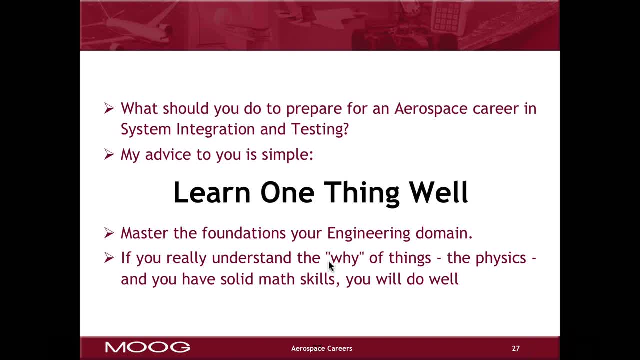 Because we want you to be very good at one thing. that will allow you to have a foundation to learn, a context for your learning, and we'll help you go to the next level. We'll help you add the important skills and the learning and growth will come as you're part of an aerospace organization. 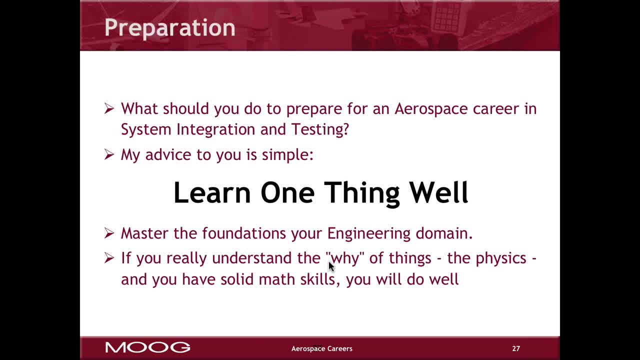 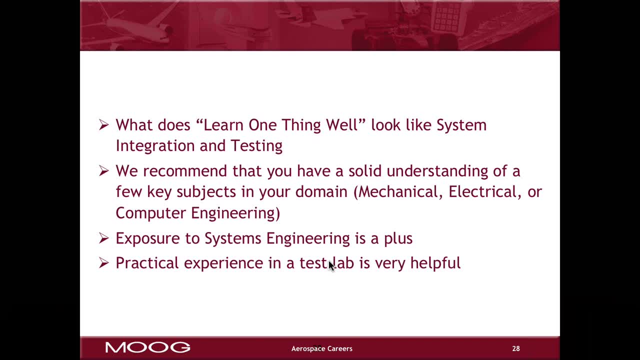 Ultimately it gets down to, you need to have an understanding of the physics, You need to understand the why. And the next slide it talks about the fact that systems engineering is a plus. We didn't talk a lot about systems engineering, but the systems engineering domain. 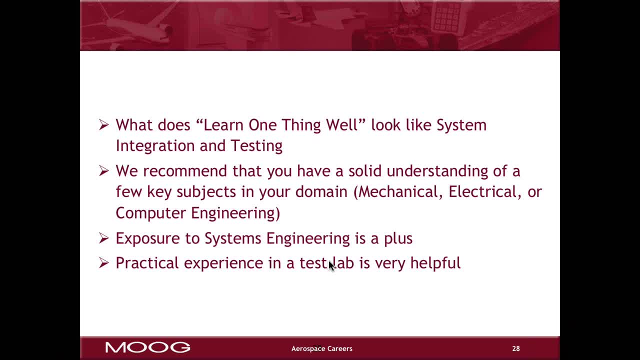 meaning the understanding of control theory and of how all of the different domains engineering disciplines work together. that's a great help, And so a basic exposure to systems engineering could be a plus, but never to distract you from your understanding of your key domain. 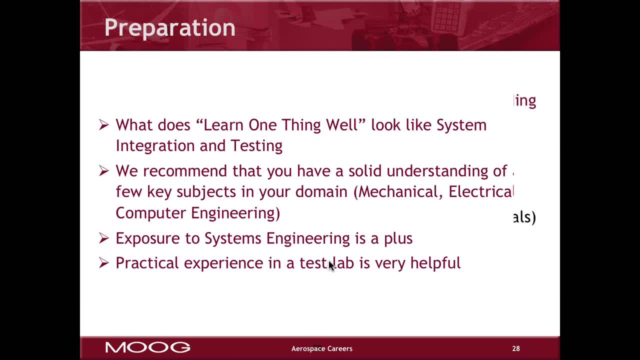 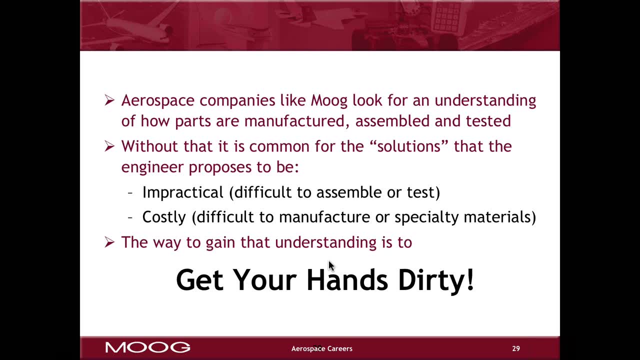 And then if you get practical experience in a test lab, that's, you know, a great, great plus. There's one other important factor for you to remember, and that's the thing that I'll say it this way: aerospace companies like Moog look for an understanding. 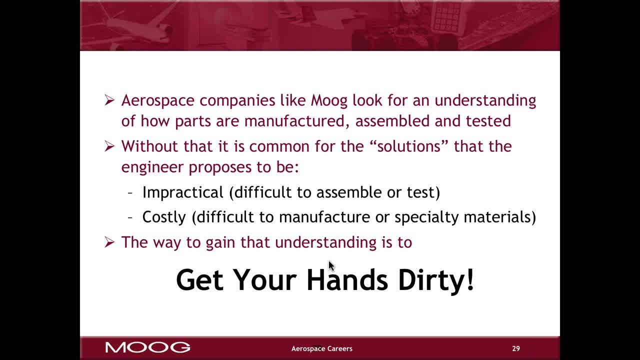 of how the parts are made, how they're manufactured, assembled and tested. We're looking for more. We're looking for more than a theoretical understanding of how to draw a circuit diagram, or how to do a finite element analysis or how to draw a logic diagram. 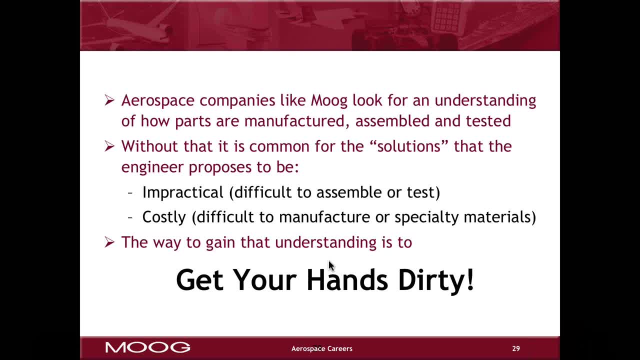 We're looking for young men and women who want to understand the solutions that are grounded in an understanding of how parts are made. Otherwise, it's easy for a young engineer to propose solutions that are either impractical because you can't assess them. 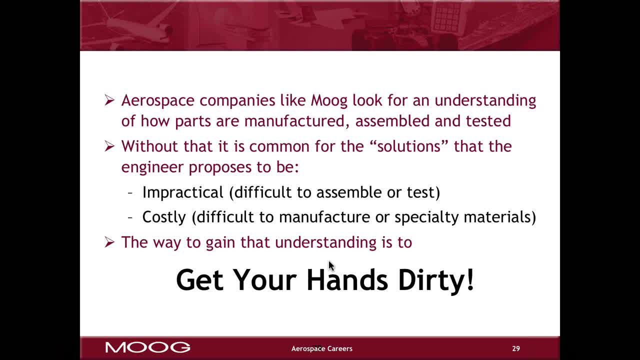 You can't assemble or test them easily or too costly, because the manufacturing methods are too costly or they use special materials that are too costly. The simple way to explain that, perhaps the best kept secret, is the way to gain real good preparation. 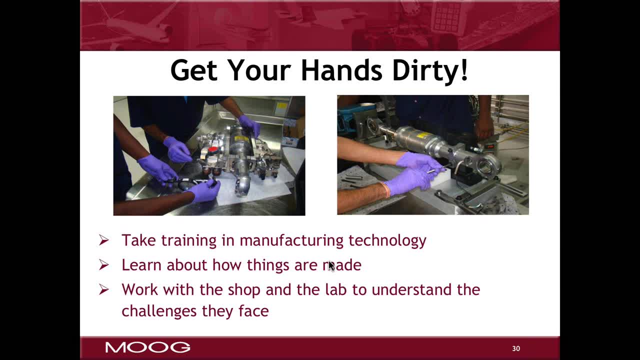 is to get your hands dirty. Don't be afraid to get into the lab or get into the lab, or get into the lab or get into the shop and actually get your hands dirty touching the parts In aerospace. we believe that getting experience with the hardware is critical. 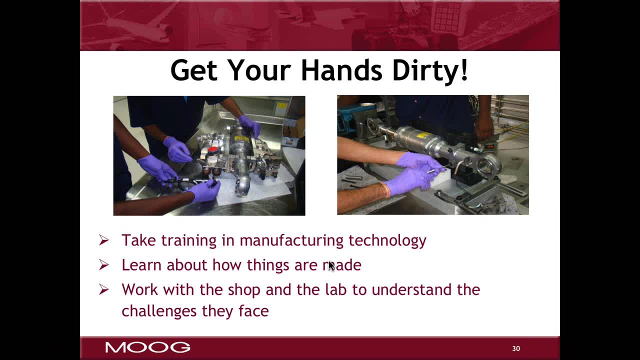 And the engineer who sits at the desk with the computer and never engages with the hardware is at a big disadvantage. We'd encourage you to take training in manufacturing technology to learn how things are made. We'd encourage you to, if every opportunity you get, to work with the shop and the lab. 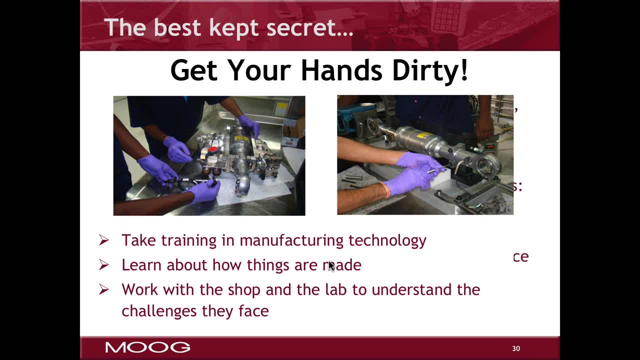 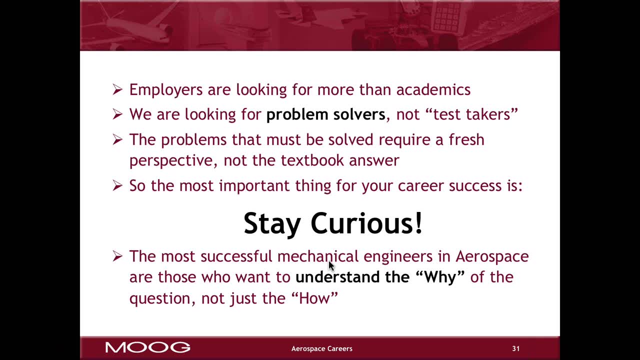 and understand the challenges that are faced there. If I were to summarize a lot of those thoughts and distill them down into just a few things, I'd say it this way: Employers are looking for more than academics. Your exams are very important. 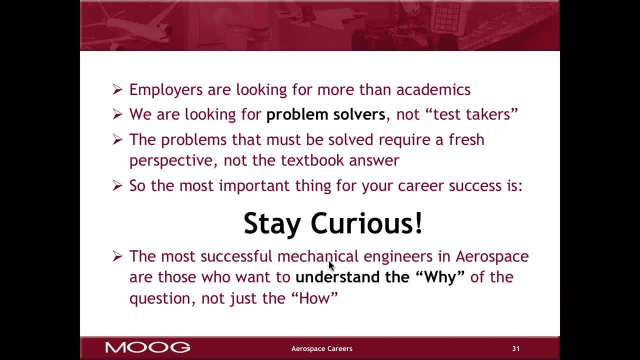 And we would expect that you'll be very good at your academic subjects And, because of the competition for joining the companies, the higher scores will actually give you a higher visibility in the recruiting process. But ultimately we're looking for problem solvers, not test takers. 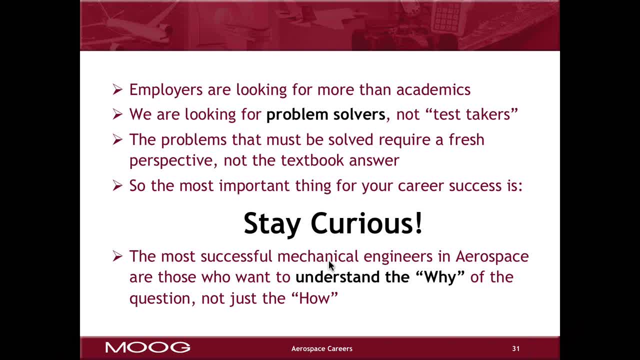 The problems that we have to solve in aerospace require a fresh perspective, not the textbook answer. So the most important thing for your career success is to stay curious. Start with the foundations and stay curious And the rest will come. The most successful mechanical engineers: 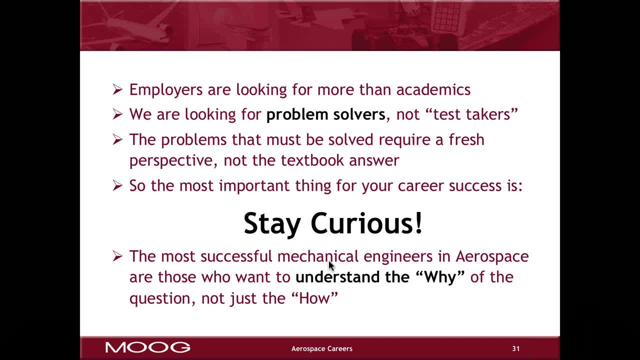 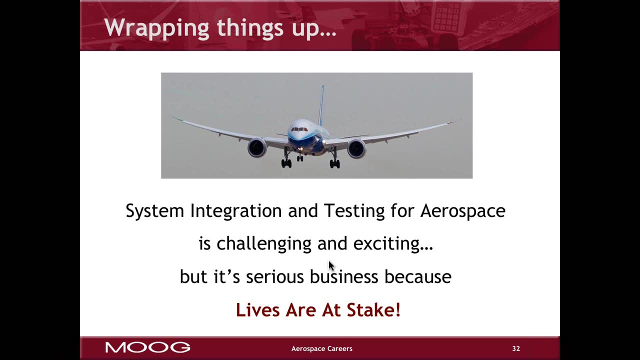 electrical engineers, computer engineers in aerospace are those who want to understand the why of the question, not just the how. The most important thing stay curious. So as we start to wrap things up here in the talk before we get to our questions. 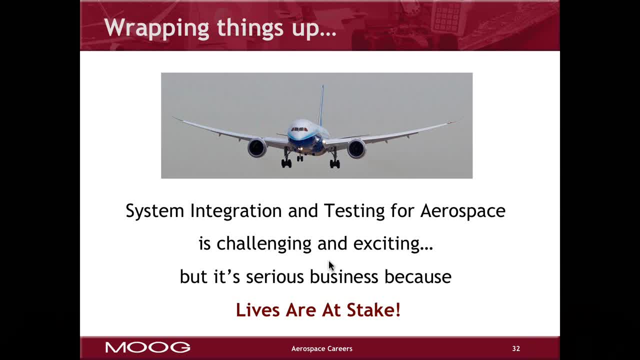 I'd like to say just a few things to remind you of where we are. I'd like to remind you of where we've been. The first part I'd like to remind you is the system integration and testing domain for aerospace is challenging and it's exciting. 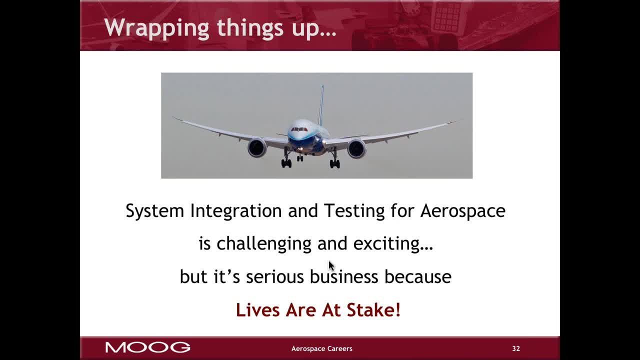 We're working on things that fly. We're working on products that go to Mars. We're working on products like UAVs and fighter, jet fighters, Commercial aircraft. All of those are exciting work, but it's a serious business because lives are at stake. 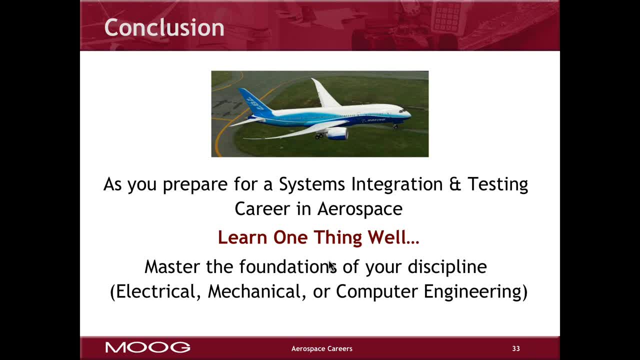 And because of that, we are very careful in choosing engineers to join aerospace. We're looking for engineers who are excited and passionate about what they do. We're looking for engineers who are passionate about what they do. We're looking for engineers who are passionate about what they do. 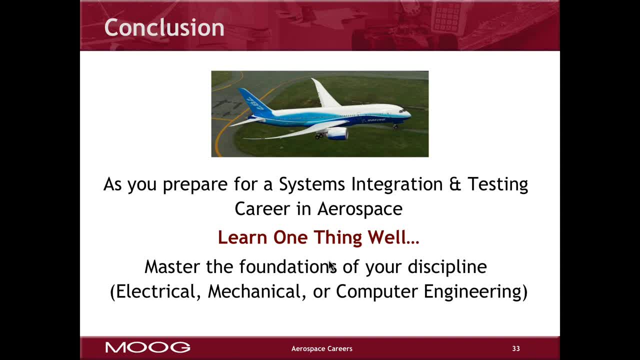 We're also looking for engineers who understand the gravity, the responsibility of what it means to design for aerospace. So, as we conclude, I would encourage you, as you prepare for, perhaps, a system integration and testing career in aerospace, I would encourage you to learn one thing well. 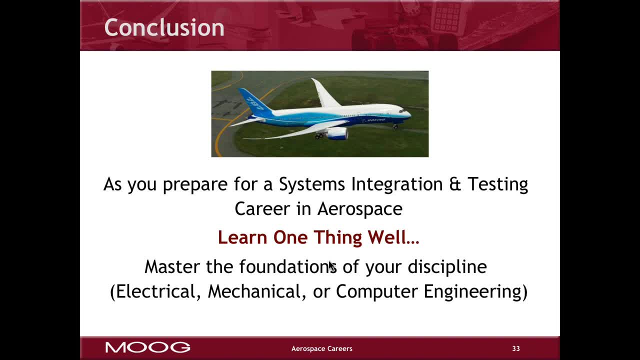 Master the foundations of your discipline. Maybe it's electrical engineering, Maybe it's mechanical, Maybe it's computer engineering. Well, you don't have to know it all when you get here. We're looking for someone who is willing to learn and wants to grow. 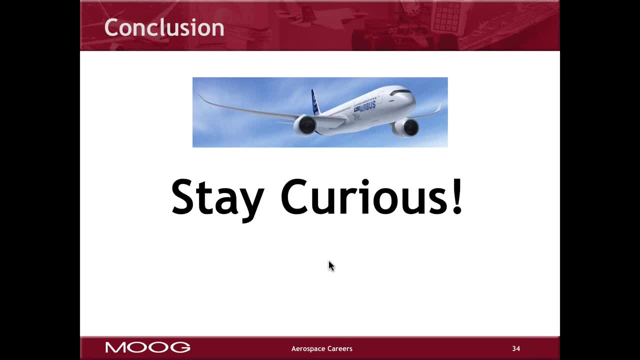 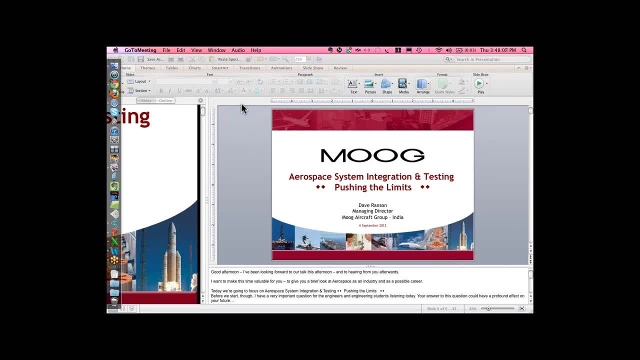 organized in their thinking. Hope that helps. So we're looking at the next question. It's an aerospace structures engineer with five years experience would like to move into system integration. The question is: does the engineer have to start as a fresher or will the experience in structures count? 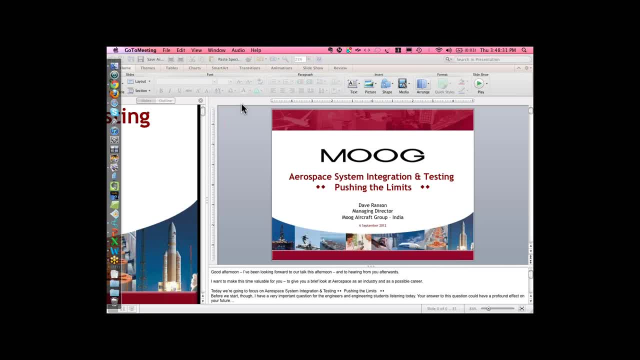 I would encourage you that your experience in structures can be very helpful in the mechanical test drift arena and then, as you worked in that arena, you could branch out into understanding the systems engineering pieces, which would very likely require you to take some classes and work in particular in the laboratory. 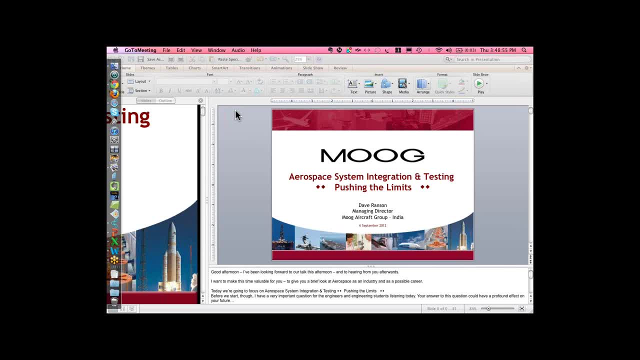 learning how to do system integration. So bottom line is: you can use your experience. it'll help you. Next question, Sujith Prasad, is asking what testing tools should an engineer be aware of for testing in aerospace? I think this is probably dependent on the aerospace company and we are. 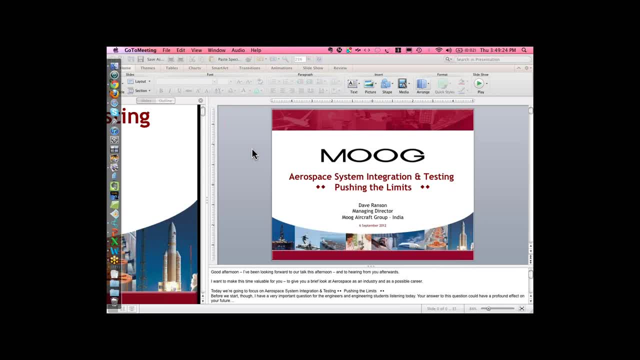 and I think other companies would be as much interested in the ability to understand the concepts of aerospace and how to use them As we would a specific tool. So, for instance, there's a large community for the National Instruments product LabVIEW and that couldn't hurt you to have that kind. 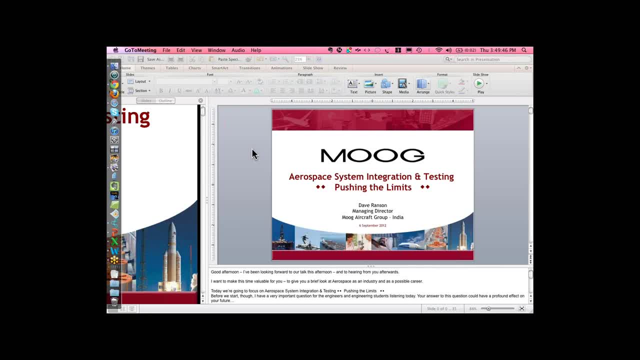 of experience, but it's not mandatory. There are other packages that do similar things. We use DSpace occasionally and first specific applications, So I wouldn't worry so much about getting a whole lot of experience in a particular testing tool. Shruti Kushik is asking. what's the difference between engineer and technicians in the aerospace team? Good question. So aerospace is in fact, I think, very unique in that there are specific capabilities that each team member brings to the team. Technicians traditionally have not gone for their BE or MTECH. 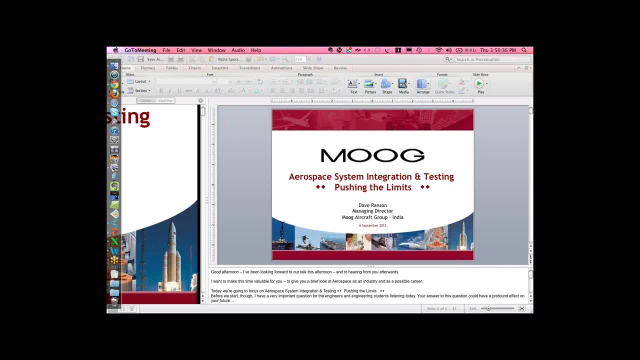 but in working with the hardware they have learned a lot about system integration and test. They've learned about instrumentation and what works and what doesn't, and so the technicians bring some practical understanding of how a system can be assembled and how a product can be tested. 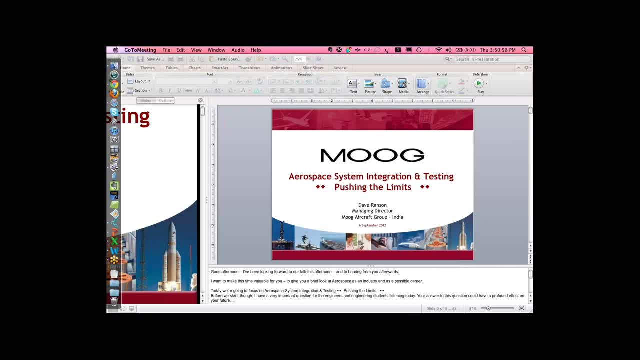 We find that the engineer- we encourage the engineer to get more practical training- Get down in the lab and work with the technician, And we encourage the technician: don't be afraid to learn the theoretical of the engineering concepts, because the more each understands of the other discipline, the more effective the team is. 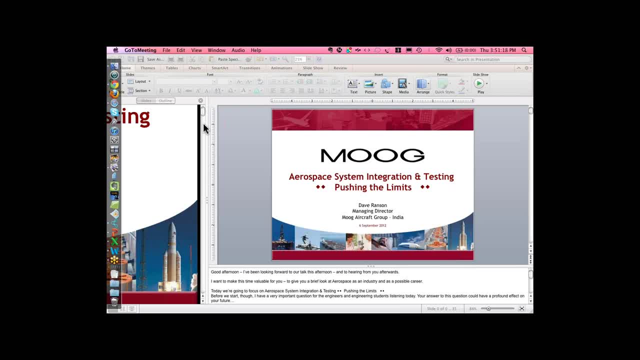 We have in aerospace companies and having been in four big aerospace companies during my career, it is very acceptable- in fact common- for some very capable technicians to assume a role of leadership in the system integration and test domain because they have such a great understanding of the practical aspects in the lab. 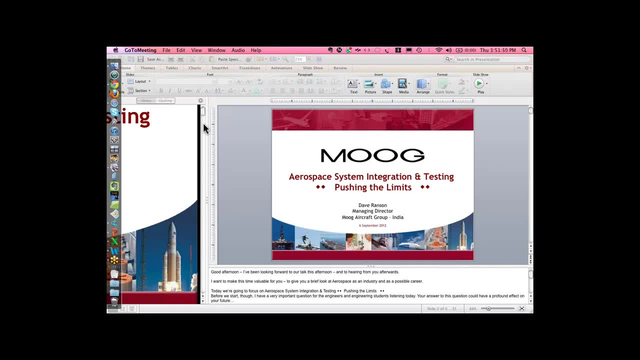 and they've learned the theoretical And they've learned to back that up and they end up being just a huge resource and very much valued. Shilpa Prashant is asking about risk management in the aerospace domain. Have we? Oh boy, that is a good question and yes, absolutely. 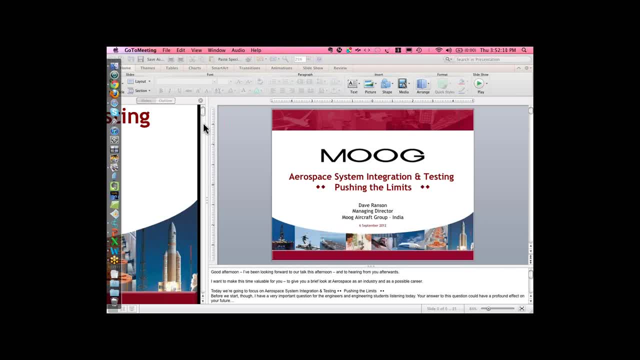 In fact, risk management has as project management, risk management has also matured significantly as a result of the aerospace world, Because there are so many unknowns in an aerospace project. If you think about the moon launches, if you think about the space shuttle launches. 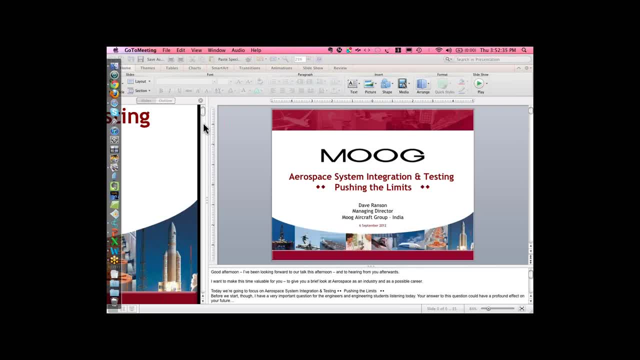 there are so many unknowns, there are so many things that can go wrong in an aerospace environment. Being able to anticipate all of those things that could go wrong, understand what the probability is that they'll happen, and then to think about the things that are going to happen- you can't do anything about it. 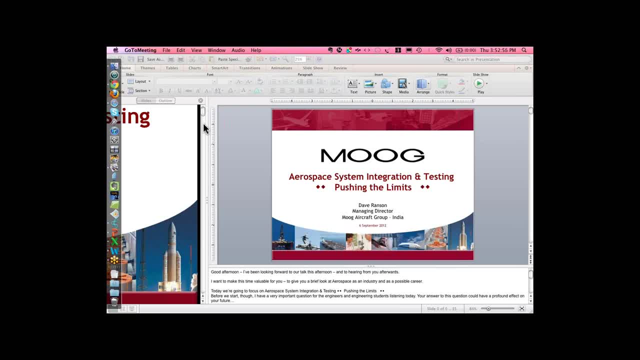 So providing strong risk mitigation actions is a critical part of our aerospace business. So your that was an insightful question. It's a very big part of aerospace. Stanley Chaka is asking what time, of what type of system integration and test facilities are available at MOG India. 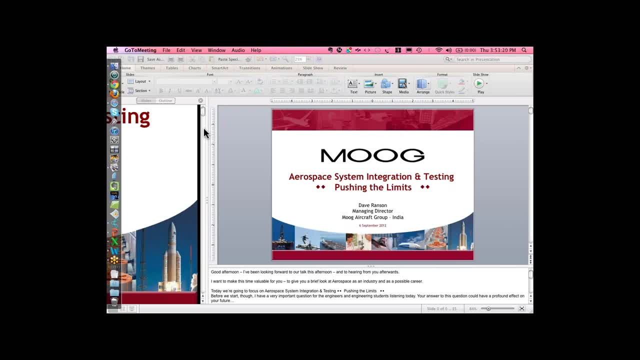 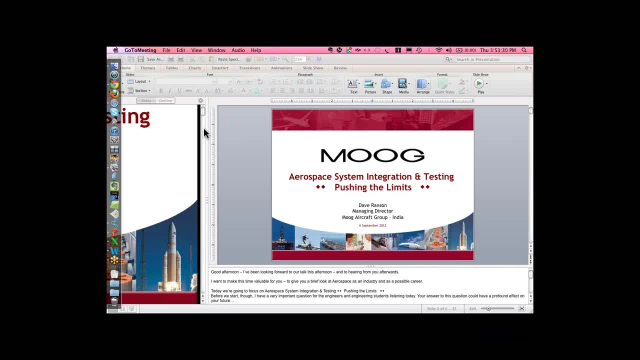 That sounds like a question from someone who knows a little about aerospace. I think there are a couple of questions there. The first one is: what type of facilities are available at Moog India? Moog has a technology center in Bangalore and we have full mechanical and electronic qualification facilities. 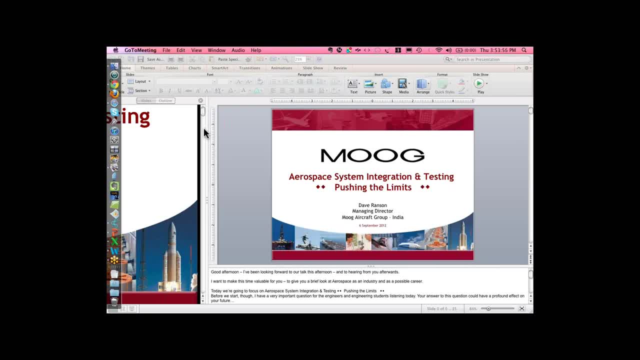 for FAA certification of commercial aircraft systems. There are still some activities that we, because of space constraints right now, will use outside labs when we get a big surge in demand. The other question is about certification. We are, in fact, participating in airworthiness and certification testing right now. 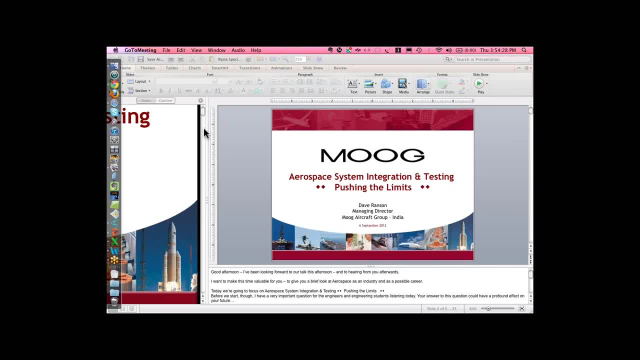 Although the BASA right now is not, we're not at a place where that's mature enough for us to use that effectively. So, for those of you who are not aware of it, basically the BASA is an agreement between the FAA and the DGCA. 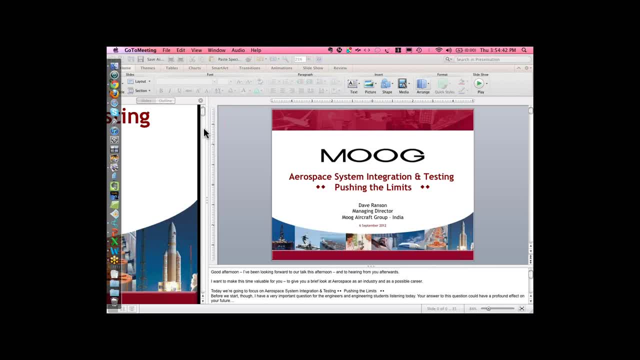 to agree to honor each other's certification efforts based on the certification. So that's a good question. That's a good question. That's a good question. We're working on some specific guidelines And that has just been signed months ago and is still to be. it hasn't been used widely yet. 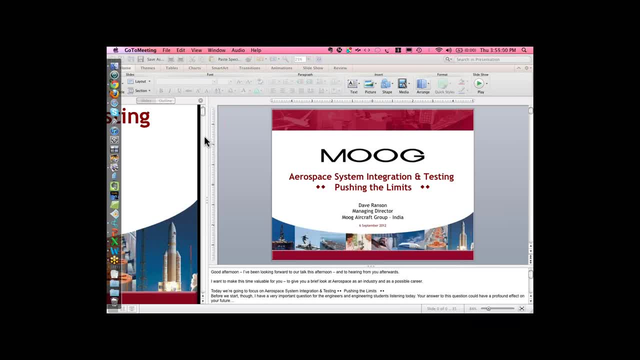 But I foresee that in our future definitely. What kind of airworthiness setup does Moog have? That's also from Stanley, So maybe I've answered it, maybe I haven't. We have a full qualification test lab here And we also have a quality department. 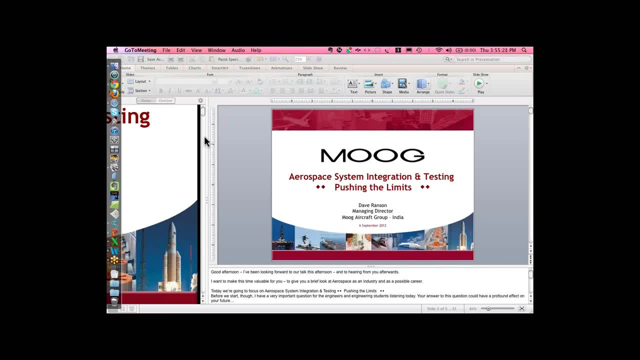 And we have trained quality personnel to oversee that And we've had major customer visits for certification activities to make sure the customers understand our capabilities And we've had good reports. Okay, Okay, Ruchikesh Sahu The question he's asking. 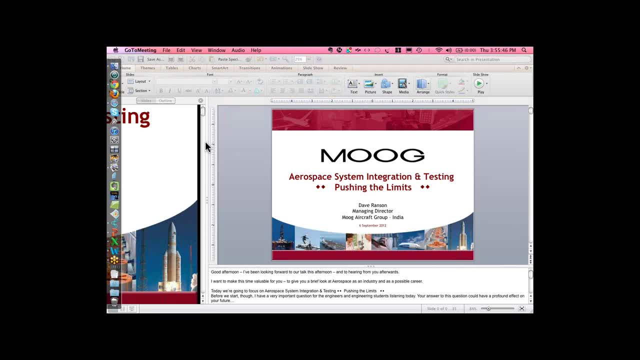 what are the disadvantages of being in the aerospace industry? Oh, there's a good question. That's a tough one. Okay, Now you have to realize this is coming from somebody who's been in the aerospace industry for 31 years, So I might be a little bit biased. 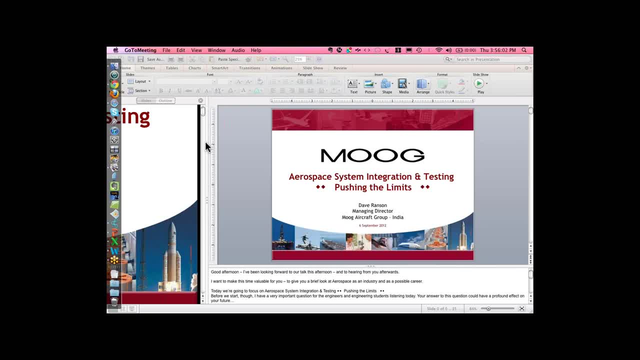 But I also might have a really good perspective, So let me see how I can help you with that. So the disadvantages of being in the aerospace industry, I would have to say it goes back to the question I asked you earlier. The question I asked you earlier is: why did you choose engineering? 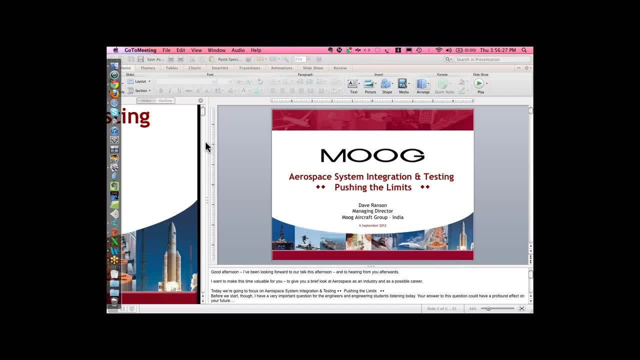 If you chose engineering because you love to solve problems, you love new technology, you love inventing things, you love the fact you can advance without becoming a manager, then aerospace is a beautiful fit. If you chose engineering because your goals are to have a very high salary, 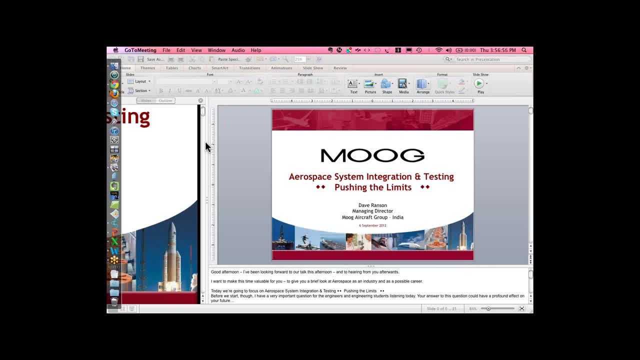 and an impressive title, which is a fine goal. if that's the reason you got into engineering- because engineering can provide that in some companies- then aerospace is not going to be as advantageous to you, because it will be slow and steady, Okay. 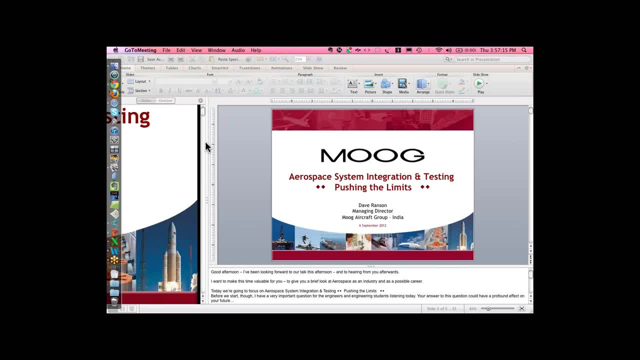 The aerospace business will. It will allow you to grow slow and steady, always earning a good income and eventually having a much higher potential in the mid-career than in engineering services, And also being able to have an established reputation for yourself internationally in aerospace. 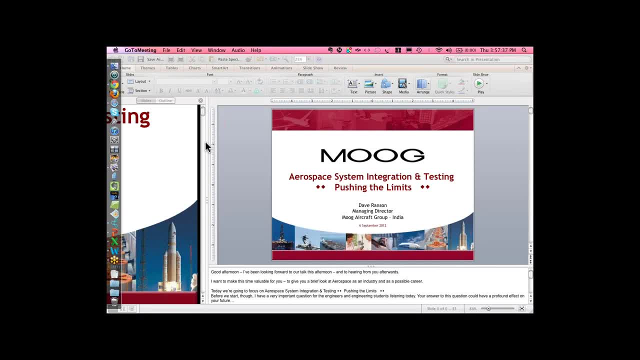 Difficult to do in some of the other sectors, where you're one of thousands. Hope that helps. Main challenges in the aerospace sector: System integration: Shulup Roshanth. Okay, Main challenges. I think the main challenge that we talked about is the one I would identify here. 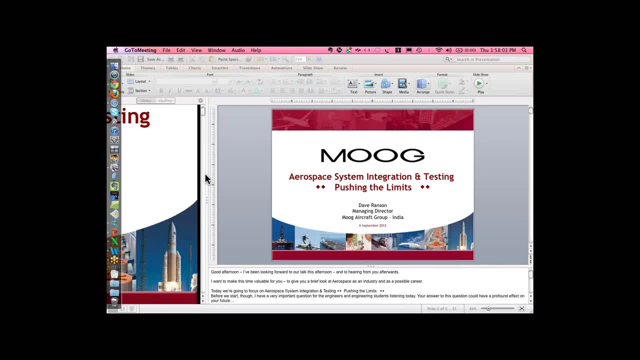 and that is being absolutely sure that we are making sound engineering decisions regarding the safety of the product, Because, ultimately, we are going to be innovative, We are going to push the limits, We're going to test. It's our job in the certification part to find out where the system will break. 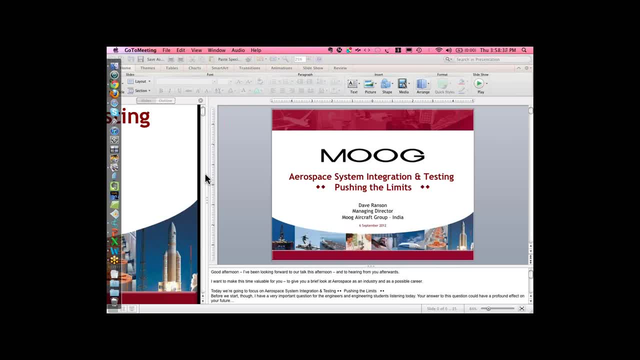 We're going to do all of those things, But the biggest challenge is making sure the product is safe And will remain safe for its entire service life. Here's another question from Ruchit Kash. And you're asking about without aircraft control. 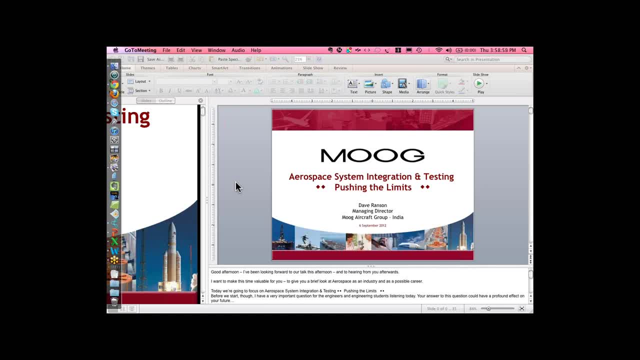 what is the minimum descent rate? you can descend the plane. Well, you found the question I can't answer. Although I do aspire to become a pilot, I have not had pilot training yet. I do know, though, that that depends on where you're descending from and what aircraft you're in. If you're at 15,000, 20,000 feet, then the descent rate is different than if you're coming from up at the higher elevations. I'll bet you could find that on the Internet. I'm not sure if you could trust the answer. 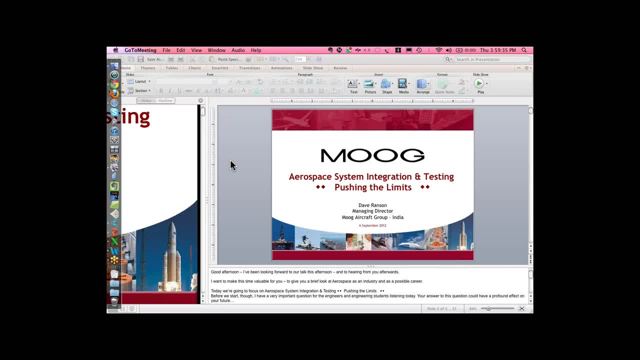 There's probably a Wikipedia article on that. Okay, This is Shalil Prashanth, again asking what type of standard used in quality assurance Of the space shuttle parts. That's a good question. I'm going to have to answer that in real, general terms. 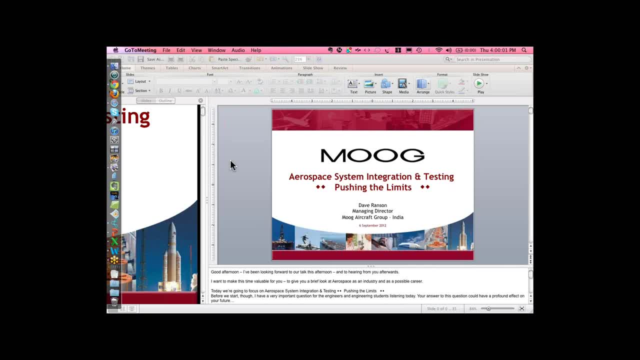 because I did not work directly on the space shuttle project. However, the quality requirements for the space shuttle were the highest requirements- And some of the other questions that were asked about risk management and project management- NASA's space shuttle program was a pioneer in several of those. 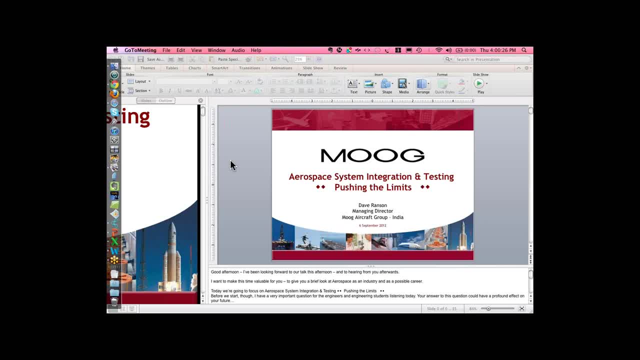 And that damaged O-ring was identified early on as a failure that was critical to flight safety and should have grounded the fleet. Just that statement there was part of an important risk mitigation risk analysis that was done by NASA for all of the potential failures, And it just points out the fact that the quality assurance system is only as good. 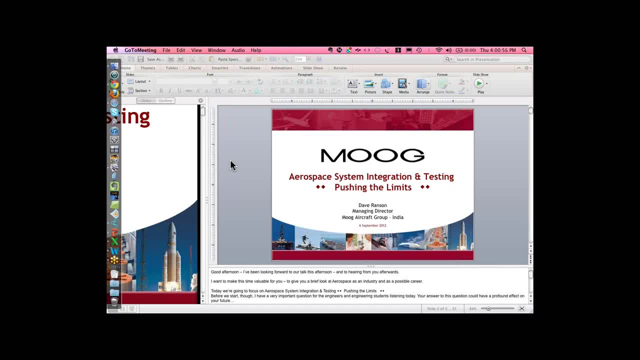 as the decisions are made by the people who are working in the system, And that's- and I need to be careful there because I have the utmost respect for thousands of engineers that worked on the space shuttle program- And that mistake in judgment that we made was a mistake that we made. 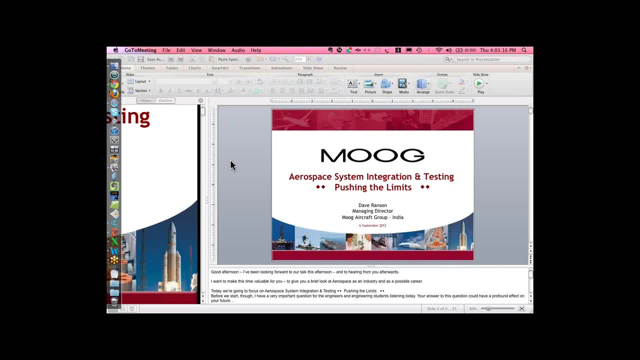 And that mistake was made by a few- should not in any way taint the reputation of the thousands of excellent engineers with absolutely top integrity who worked on the space shuttle program. Okay, here's a good question: How many levels of testings are needed in aircraft launch? 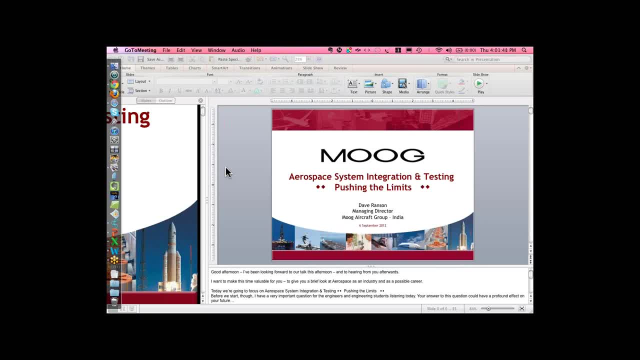 I'm going to have to tell you only the part that I'm familiar with, And that is the part that is related to the systems and the hardware that an aerospace company, what we call the tier one company, provided to the main companies that are building the actual aircraft. 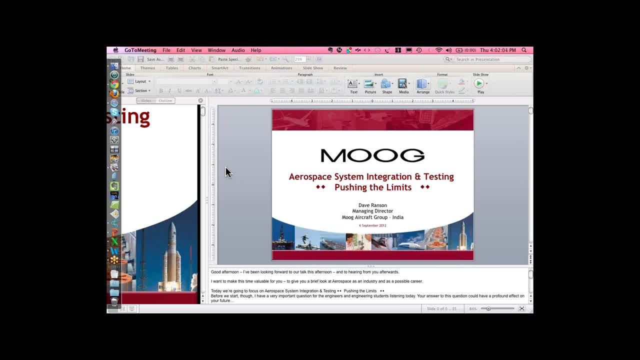 So MOG is a tier one supplier to Boeing, to Lockheed, to Northrop Grumman, to Airbus, And so we don't have visibility of that. We have all of the testing that happens prior to launch. I'm assuming you're talking in terms here of a space launch. 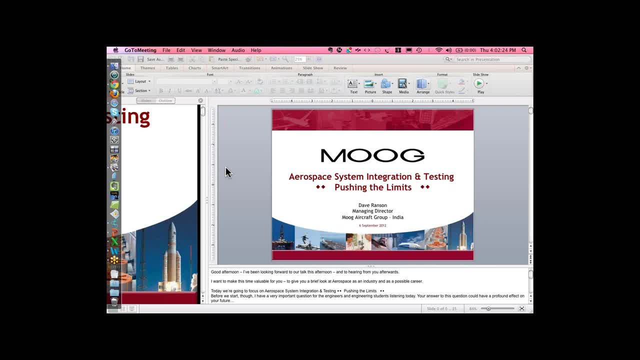 And whether it's space or aircraft. at an aerospace company like MOG there are several levels of testing. First, individual testing of small component pieces that are before they're assembled on a larger actuator. Then there's actuator level testing. 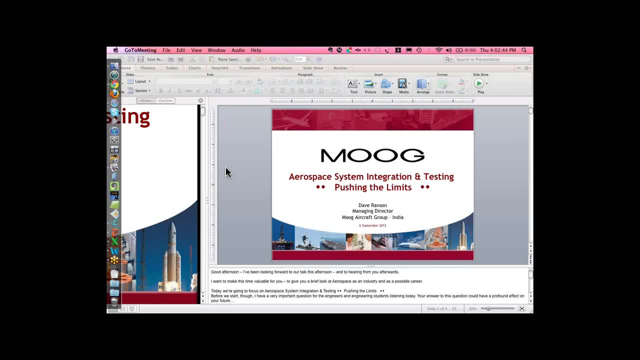 And then there's what, what, what would call subsystem level testing, where the computer and the actuator, whether it's gears or hydraulics, and all of the cables connecting them, are tested to make sure that they perform both as quickly as expected. 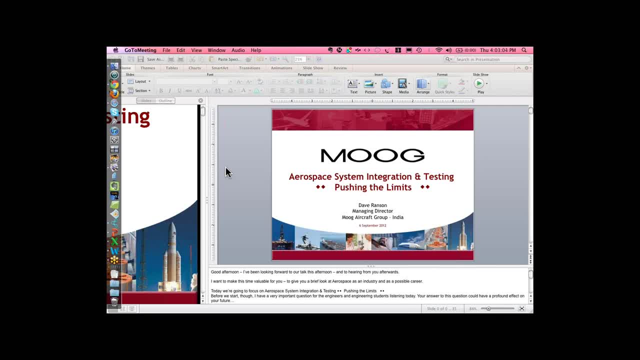 and also that they last as long as expected. Hope that helps. So there are a good four levels of testing that happen before the parts even get to a company like Lockheed And certainly before they get on to the launch pad. Next question: In the present international market, 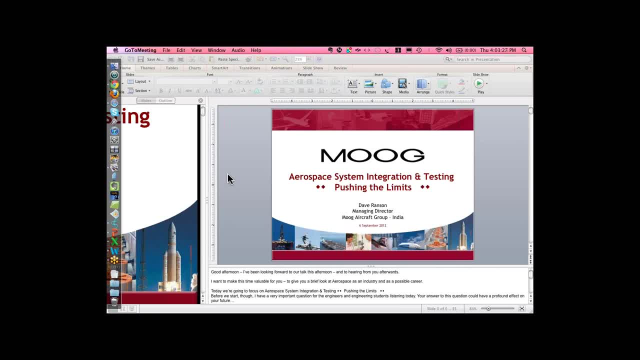 especially in the Indian market. who are MOG's competitors? I can tell you a few, because it's a small community, but it depends on what market we're in, And so I can tell you: in aircraft, United Technologies has several of their subsidiaries that compete directly with us. 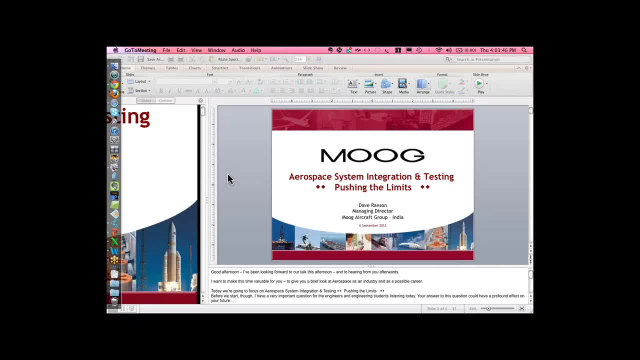 There's a company in Europe called Libere that competes with us in some cases. There's a company called Parker Hannafin that competes with us. Yeah, So those are the kinds of names that you'll typically see building the kind of 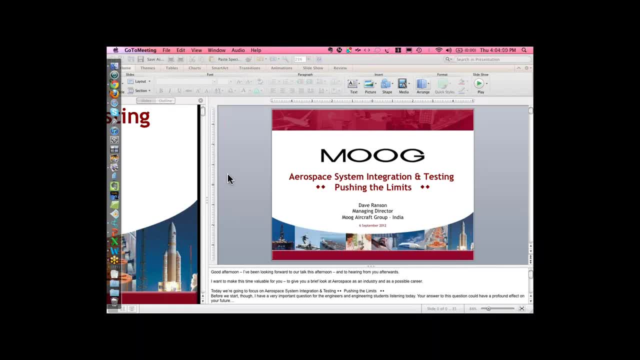 hardware that we build. We're on just about every aircraft in the West that's flying today. Next one is from Stanley. Please elaborate current aircraft projects that MOG and you is currently involved. Okay, Well, I can tell you a couple. 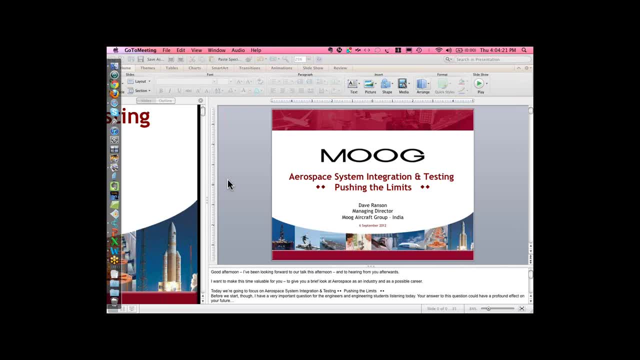 I can't tell you all of them, but I can tell you a couple of them. We are involved in the A350, and we also are involved in the Boeing 787.. There are several other programs going on here too, But, as you can understand, 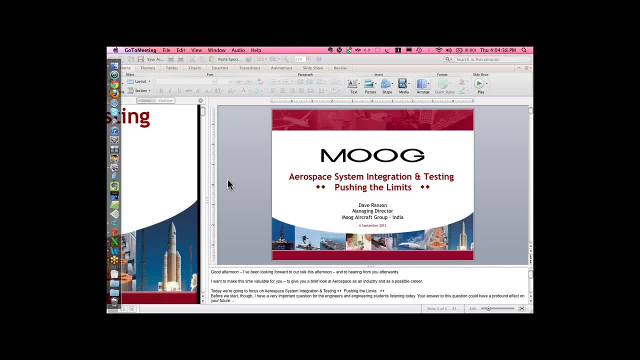 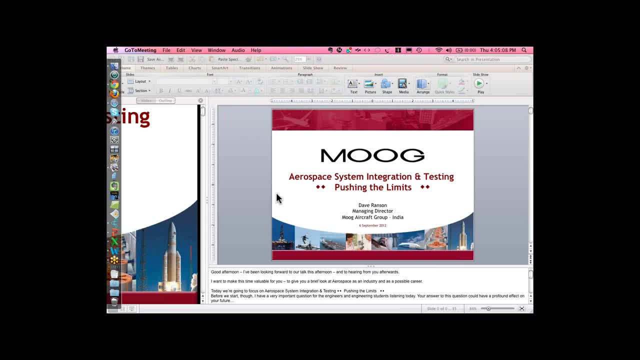 those who have tuned in that the aerospace business offers. it offers you some unique opportunities And I'd love to. I'd love to continue the dialogue. You can follow me on Twitter, Dave underscore Ransom, And you know we can continue the conversation. 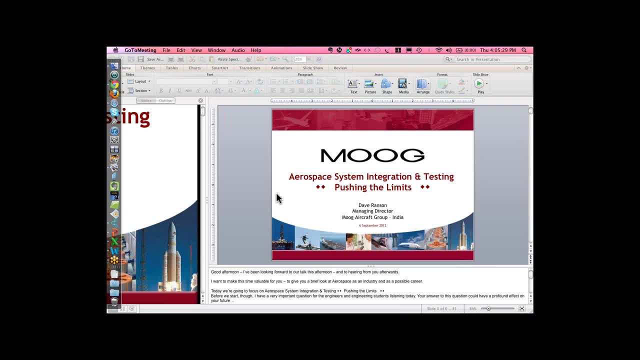 I guess we're ready to hand it back to our moderator. All right, Thanks, Mr Ransom, for your session on aerospace system integration and testing pushing the limits. It was indeed a great session. I would also like to thank all the participants for the support. 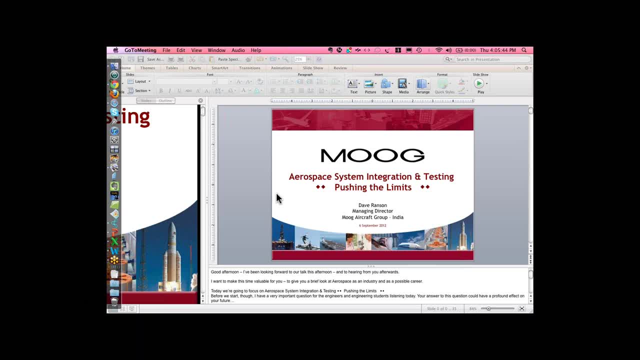 and making this webinar a success. The recording of the webinar will be available on techgeekcom by tomorrow. Thank you all once again for the great session. Thank you, Mr Dave Ransom, Have a good day And thank you for moderating. 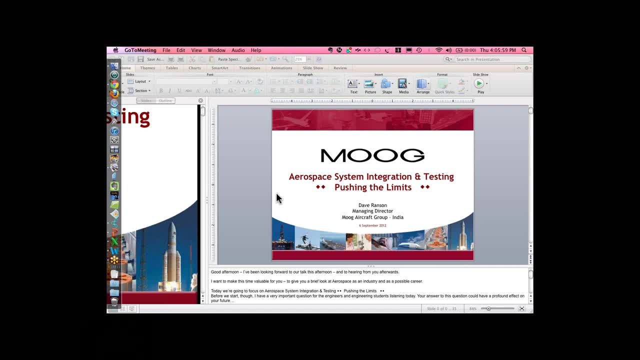 Thank you for moderating. You did a wonderful job. Thank you, guests, for the great questions. Look forward to crossing paths with you in the future. All right, Thanks, Have a great day. Have a great day.